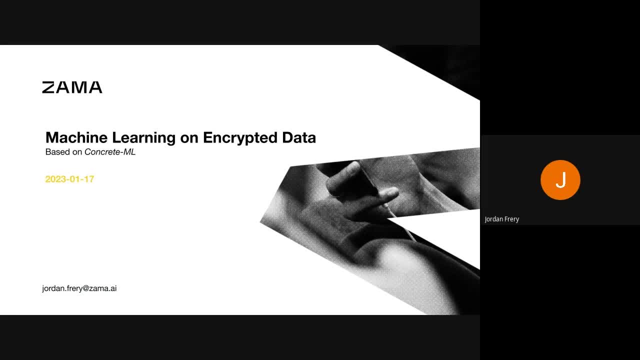 system for detection. So today I'm going to present you an open source library that we developed around the core product of Zama, which is a library that does fully homomorphic encryption, And this open source library is essentially doing machine learning on encrypted data using the homomorphic encryption. 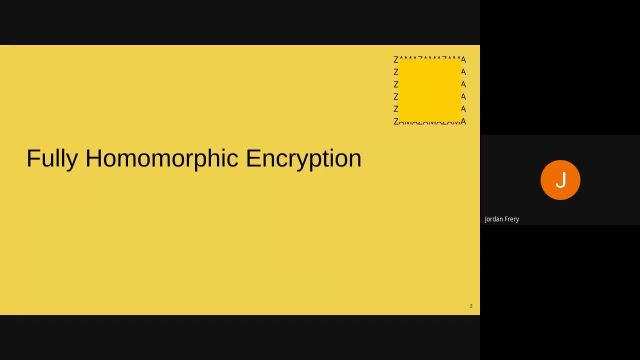 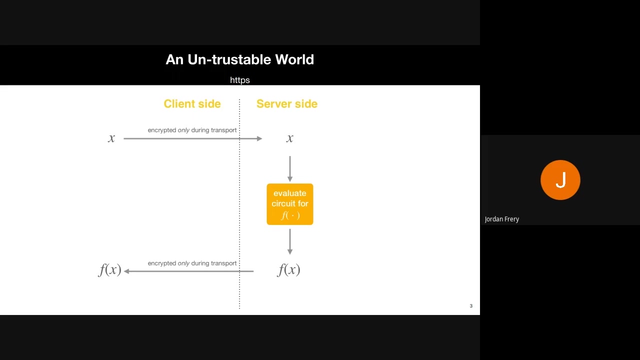 So to give a brief overview of fully homomorphic encryption, just a small disclaimer: I'm from the machine learning domain, so I'm going to give the overview here and I'll try to answer the questions you have. So currently we live in a, let's say, a stable world where 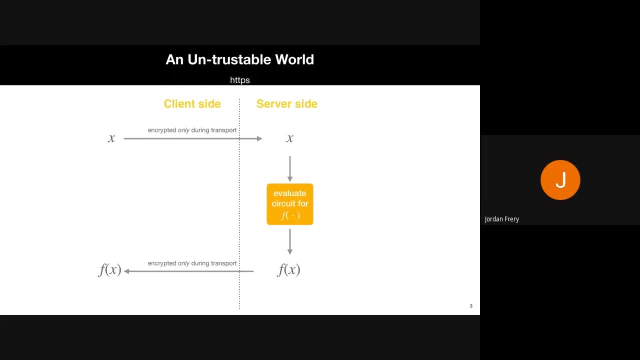 a client is able to do a lot of things. So, for example, if you have a client that is a server, you have to kind of set up a trust such that the client can get some service from a third party, a server. Let's say you send something like a mail to a server and 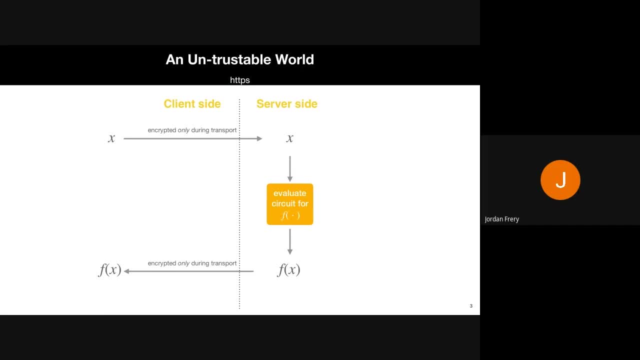 you want the server to basically do the spam detection algorithm over the mail, Since it's a complicated task, you often don't do this locally, so you just send the mail to the server. You've got to send the whole clear text to the server And the server executes the algorithm. 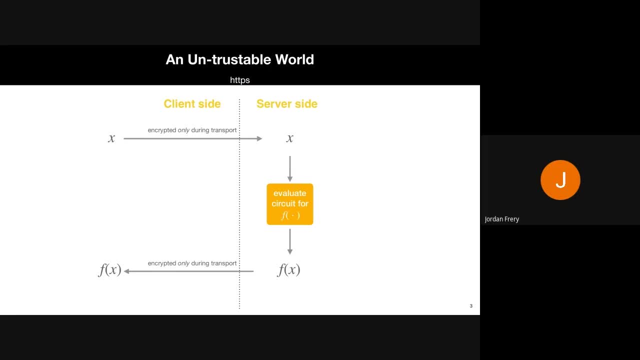 to detect whether it's spam and it sends you back the prediction or the probability of the mail to be a spam or not. So of course there is a bit of a problem here, since there is some kind of trust that is implied, because the server not only has access to the information. 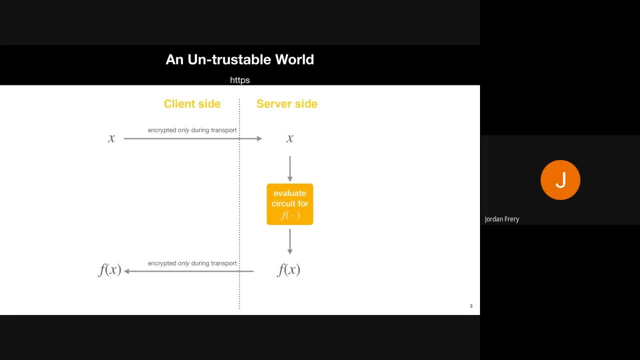 your mail, but also has access to the prediction, which basically gives a lot of information about the client. So what is FHE? FHE aims at providing a privacy for the user. So what happens is that- let's take the spam detection example again- You take the mail. you would encrypt the mail. 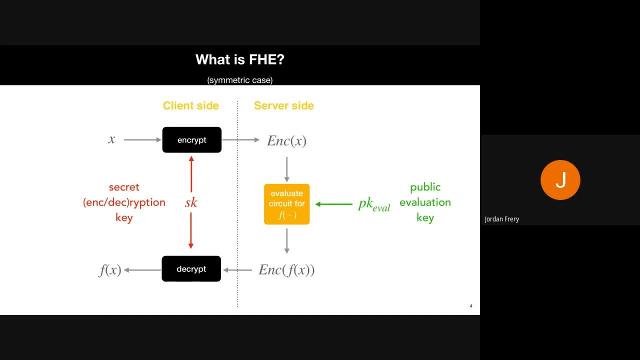 locally at the client machine and you would send this encrypted data point to the server and the server, thanks to fully-omorphic encryption, would be able to execute the same function as it would have done on the clear data and sends you back the encrypted results, Of course. 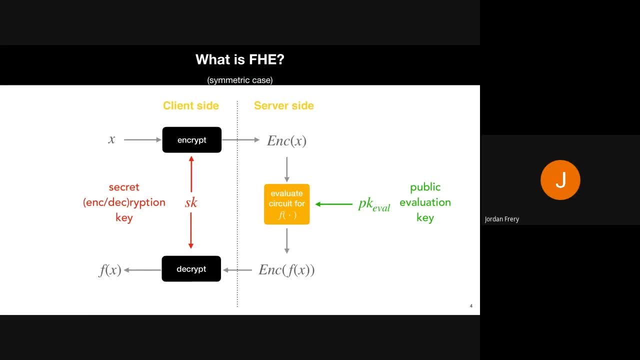 it applies the function over the encrypted data. The result of this function is also encrypted and only the client which has access to the private key which it used to encrypt the data, can decrypt the results of the function that has been executed on the server right. 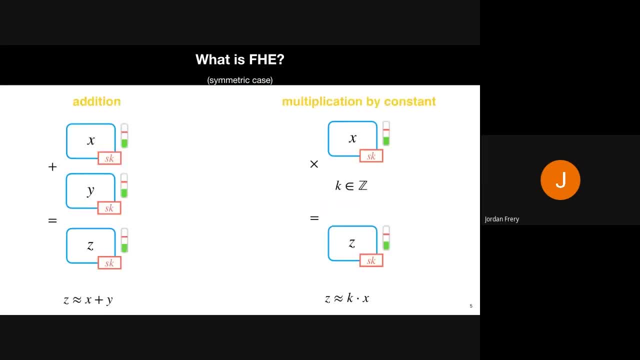 So let's dig a bit more into FHE. Here you are represented: X and Y, which can be two data that have been encrypted with a specific private key In FHE to maintain the security. you have some noise in what's called the ciphertext. 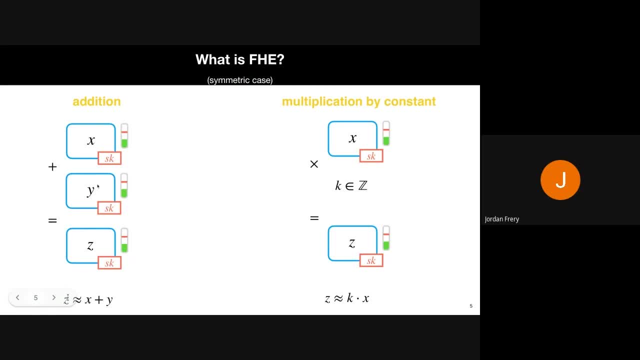 So the encrypted X and the encrypted Y, you have some noise, which here is represented by the green level here. So when you add them together, so two ciphertexts together, you increase very slightly the noise. So if you would do a very long sum, 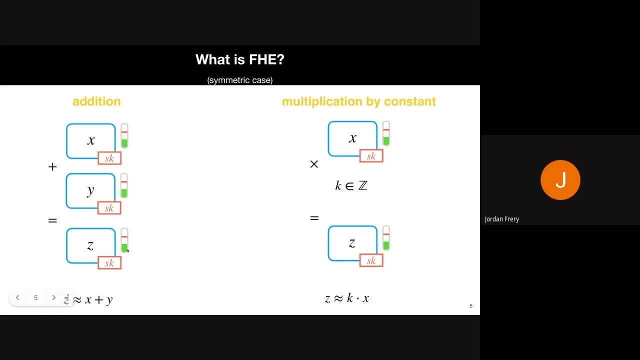 it would increase more, but so this is how adding operation FHE works. So you would adding arithmetic operation between two ciphertexts would increase a bit the noise, but that's not too bad here. for the addition With the multiplication, same thing. 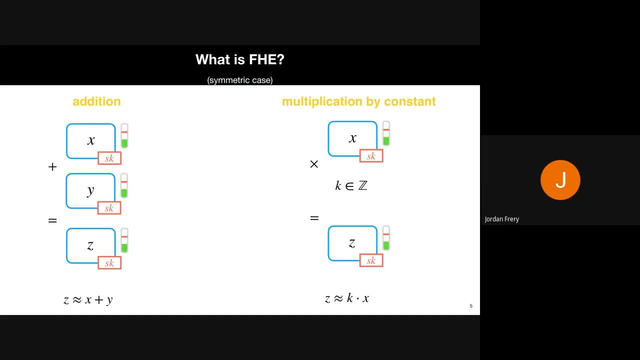 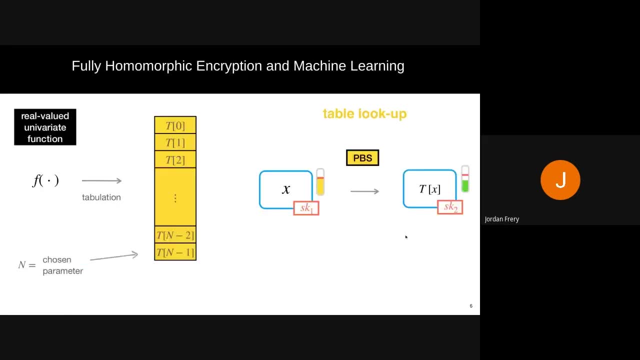 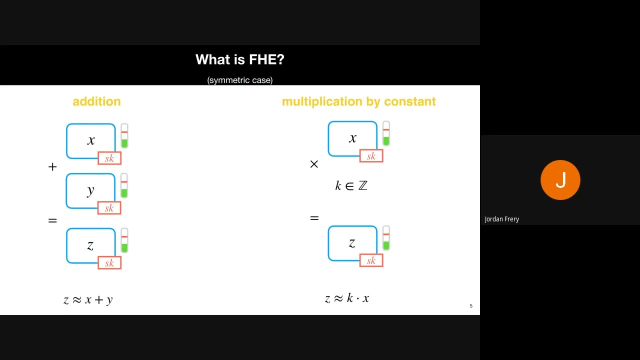 If you multiply a ciphertext with a constant, the noise remain kind of stable. So what I mean by stable is that once the noise reached this red level here, what happens is that- oops, what happens is that then the noise is basically overwriting. 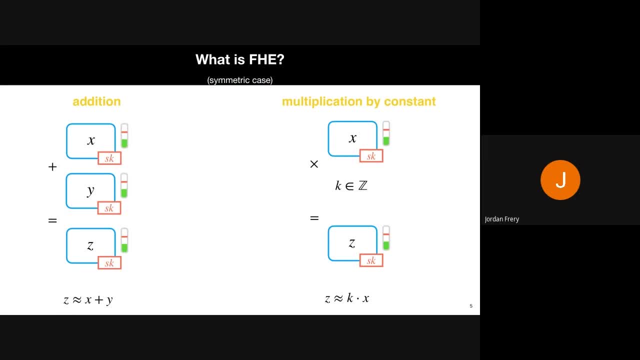 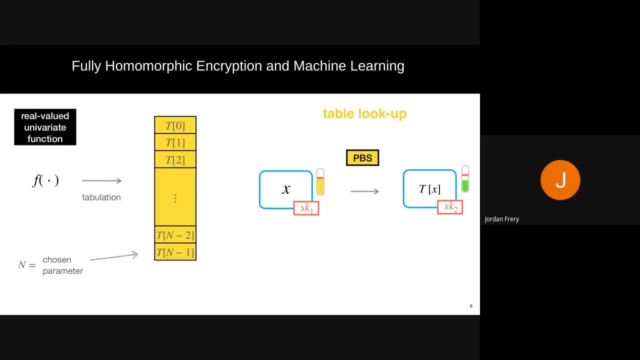 like the actual data that has been stored in the ciphertext. So when you do a lot of computation you will arrive to a point where the noise is quite high. So in fully homomorphic encryption there is something called a programmable bootstrapping. 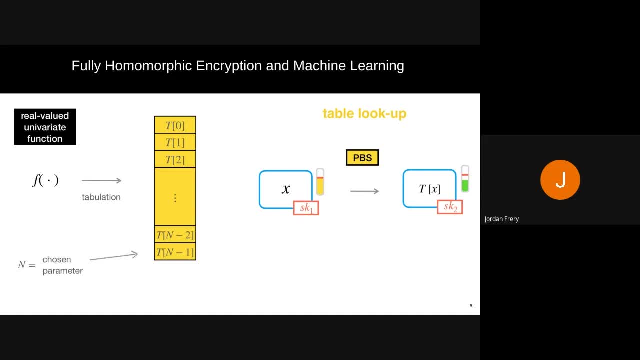 which you call here PBS. At our level, at the machine learning level, this programmable bootstrapping can be seen as a simple table lookup, So essentially just mapping any variate function from an integer to an integer, to another integer right. 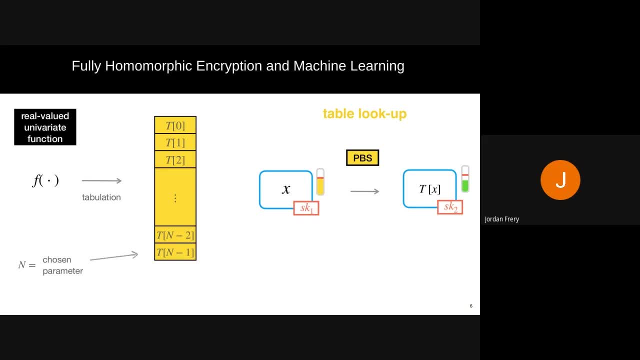 And this is quite interesting because this table lookup allows us to have some kind of non-linearity in the FHE circuit- but also, when you apply a PBS, it decreases the noise, So you can keep working with this ciphertext that comes right after the PBS. 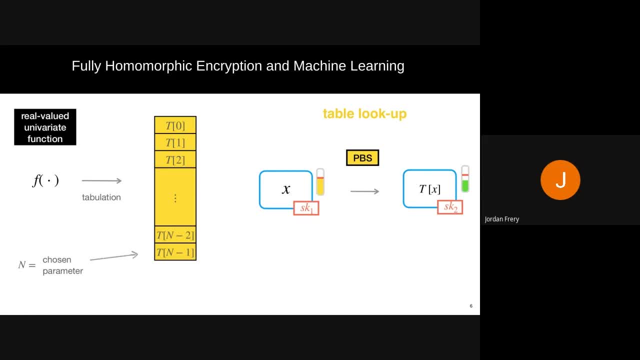 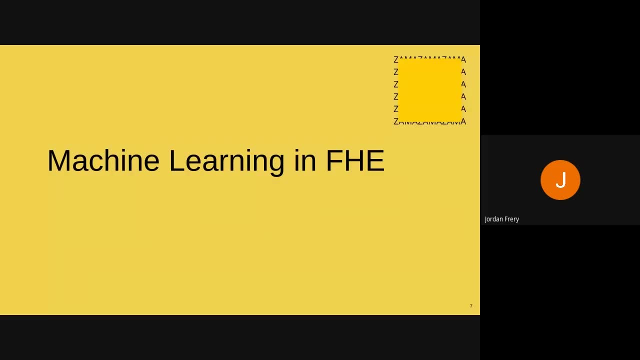 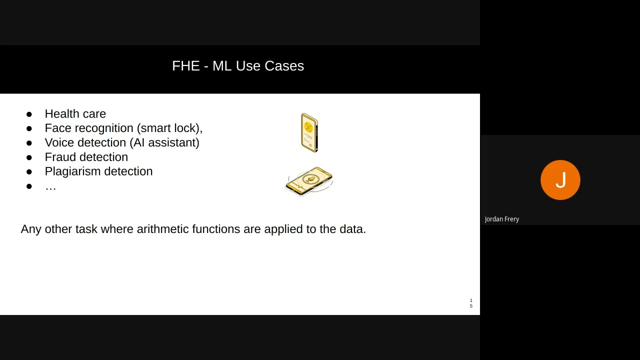 So this is why machine learning becomes very interesting in this case, because you could have very long circuits and always play around these PBSes to decrease the noise and keep going with the computations. So let's tackle a bit more machine learning use cases here. 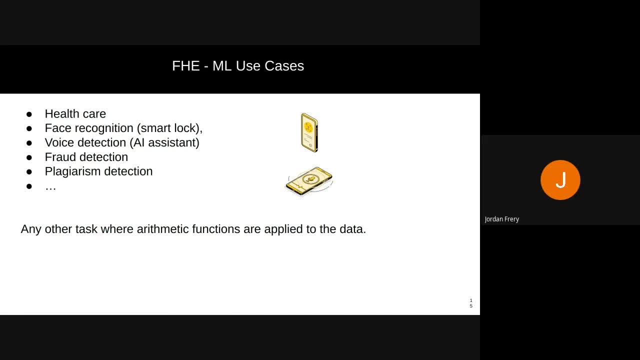 So, of course, the first one that comes to mind is based on how do you use this? It's based on healthcare, where machine learning is a bit stuck today because of obvious reasons of data being very sensible to share and compromises some privacy from the users. 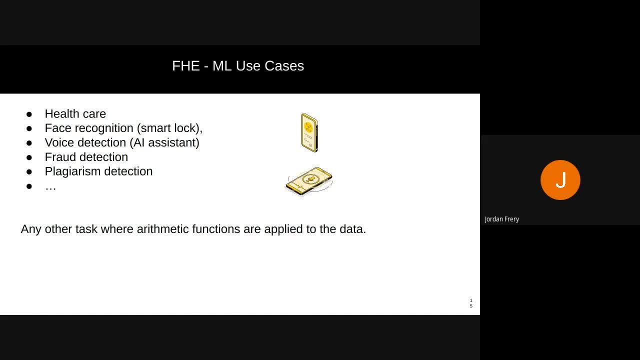 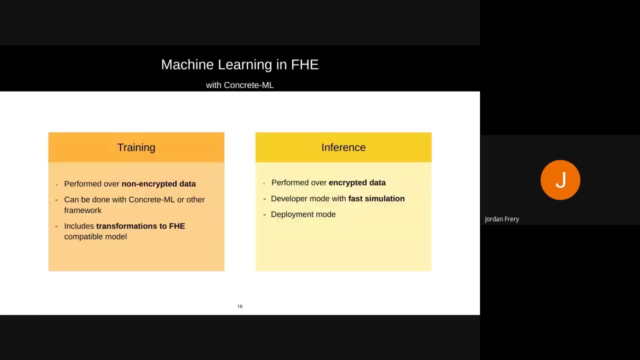 Of course there are a lot of different applications that can be done, like face recognition, voice detection, fraud detection, basically any arithmetic functions. So all the different applications, all the different types of analytics that can- that represents machine learning models- can be done in FHE. 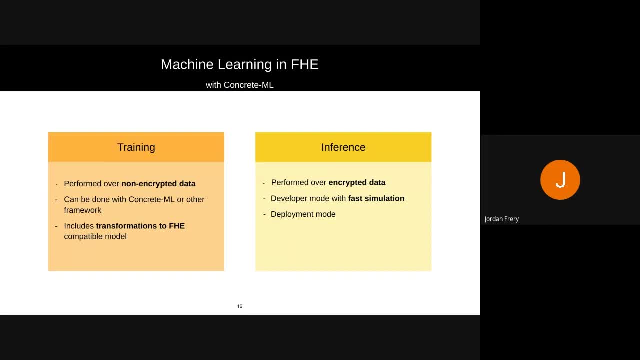 So machine learning, currently, with the fully homomorphic encryption that we have, now we are performing the training of the machine learning model on non encrypted data. It can be done with the open source library I'm going to present right after, be done with anything you'd like, and the library is supposed to convert any machine learning model. 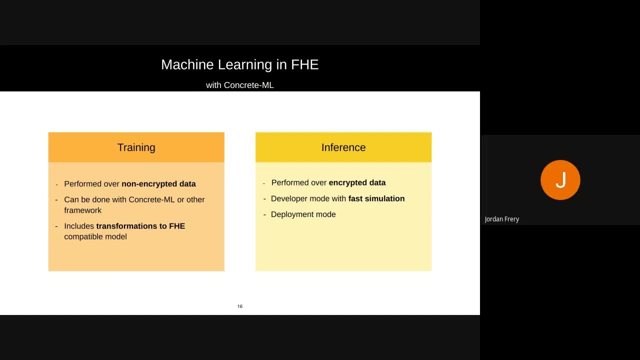 to its fhe equivalent and the. the pros of concrete ml for now is to allow the inference on encrypted data. so you could train your model um. pass this to concrete ml and you would get an fhe circuit which is with the, the crypto parameters to encrypt the data. so you would. 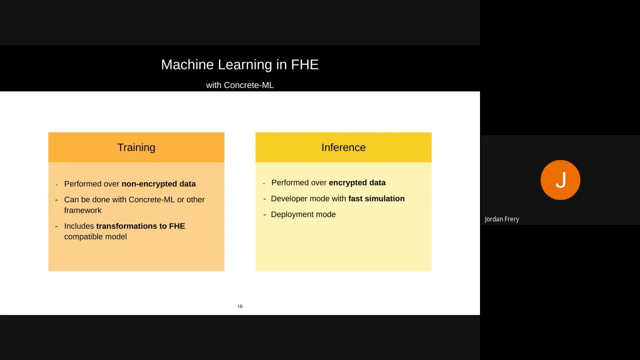 have to create private key as a client. you would have to uh, the secret key as well, and um, and then you could deploy the fhe circuit in a untrusted server which would run the inference of encrypted data. so we provide also in this library the, the fast simulation and the deployment. 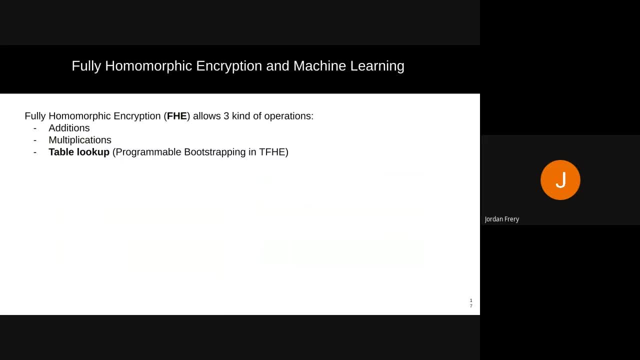 mode. uh, i might come back to this later. so fully homomorphic encryption, uh, as just said, basically imply three kind of operations, so additions, multiplications and this programmable bootstrapping which for us is going to be a table lookup, a very simple table lookup, and in machine learning, what you would get is matrix multiplications, which represents 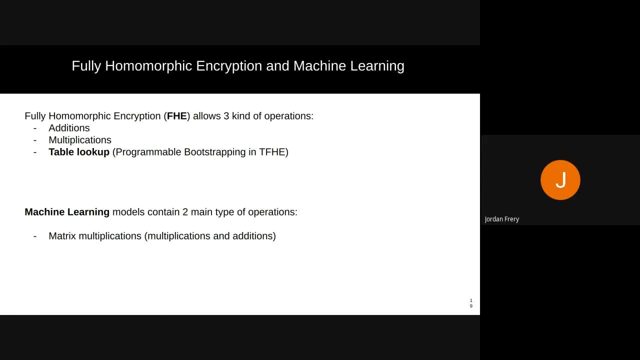 like more than 90 of all the operations you actually do um in machine learning models. so multiplication and additions, those are pretty fine to do in in a morphic encryption. and the second part is non-linearities. so in neural nets, for example, you want to break the. 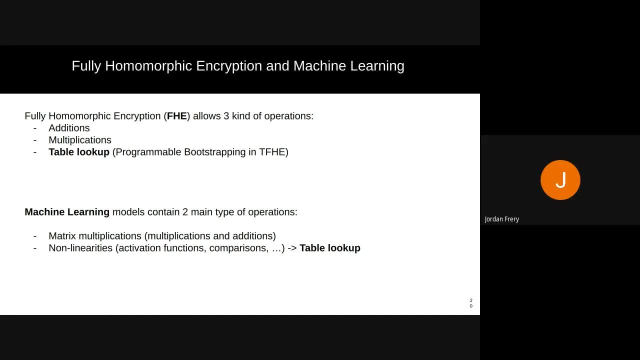 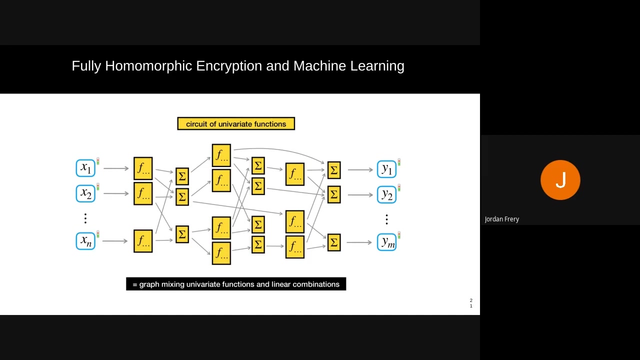 linearity by adding some activation function, non-linear automation functions. you could also have, as we will see, in trees. you have some comparisons between values. that breaks the linearity and this is going to be represented using a table lookup. so overall, fully homomorphic encryption and machine learning can be matched by having two kind of main operations. so you have the ciphertext. 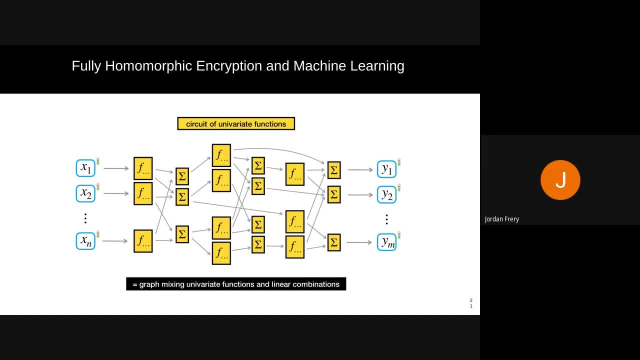 so encoded and code encrypted inputs. that comes in the machine learning model that can do whatever kind of computation it needs to be done. so here the function represents the pbs's. so those could be, you know, linear activation and you want in fhe to represent that. the them with a table lookup. the sum would be just. 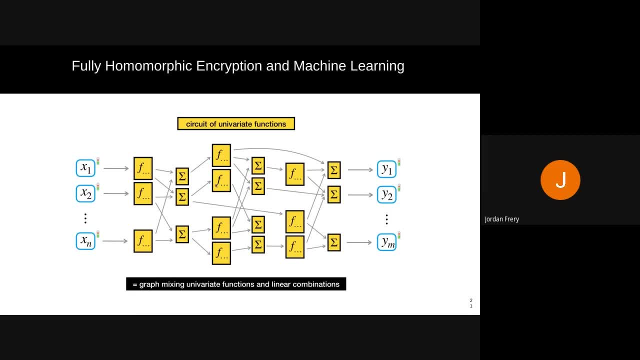 you know matrix multiplication, and then you can, thanks to the PBS's, so the functions here- you would be able to go very deep without actually destroying the ciphertext because of this noise increasing, since you can actually use the bootstrapping to decrease the noise step by step. 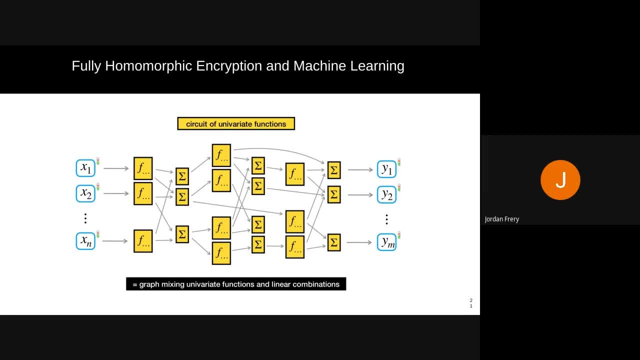 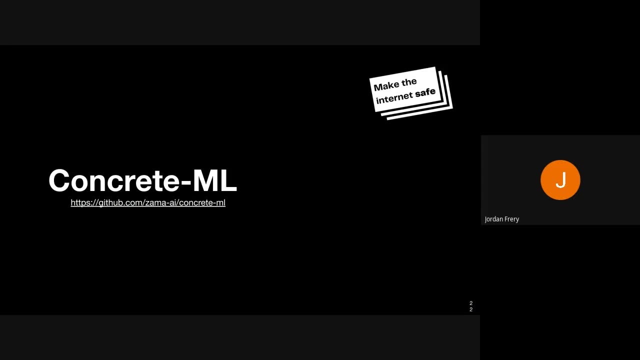 In neural nets. these PBSs happen at every level, often at every level. So after matrix multiplications, convolutions and things like that. So we have a lot of time to do that. I will leave that up to you guys to see if you have questions. 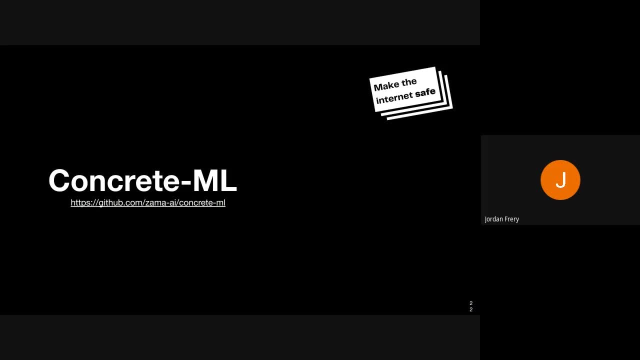 So if you have anything that you'd like to share, please leave a comment And we'll do that. So thank you very much for your time Great. So now let's have a look at ConcreteML. So it's available on GitHub publicly. 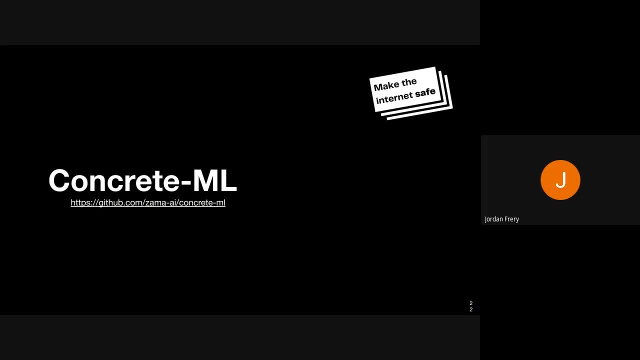 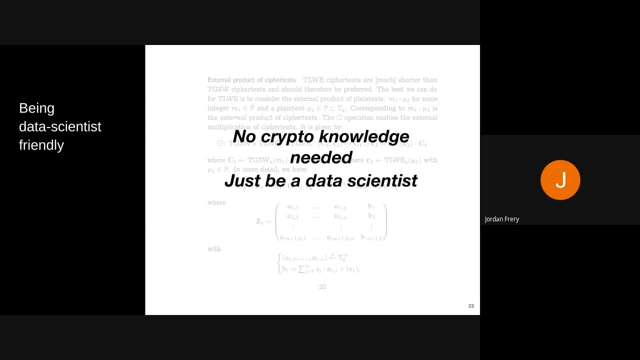 We are trying to release every three months updates As we are working with the research teams, So you can check it out on GitHub. This library has been designed so that people with absolutely no crypto knowledge could actually use it. The only thing that will be needed to know is that you have to create keys and 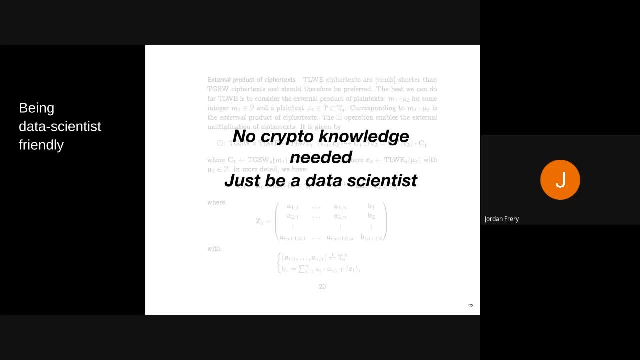 But basically training the model and deploying would be very simple. here We try to be as close as possible as what data scientists and machine learning practitioners are used to have. So in those areas like we support Torch and TensorFlow, But also all the models. 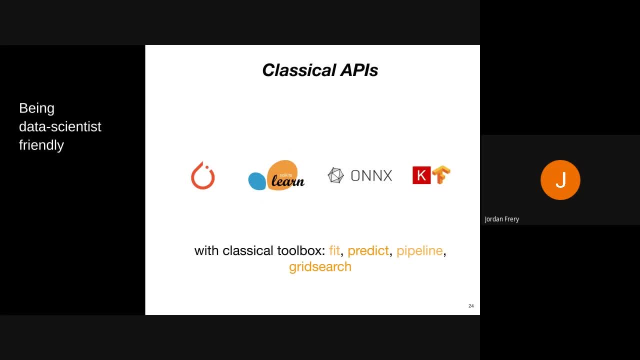 Most of the models that are available in a circuit learn And ONNX. it's a representation of machine learning models using kind of a graph abstraction And it turns out that most of the machine learning framework can be converted. model can be converted to ONNX, which is the main entry point to the learning model. 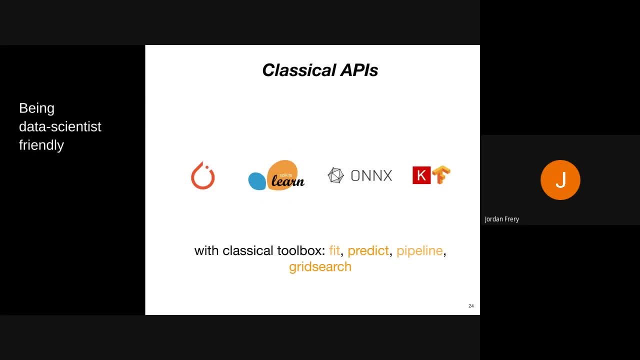 And then of course, we have the other popular API that you can have in Python when you work in machine learning with the feeds, training a model, predict others and data, And you have some pipeline and grid search also supports. So now let's dig in how we actually change the machine learning model to make it FHE. 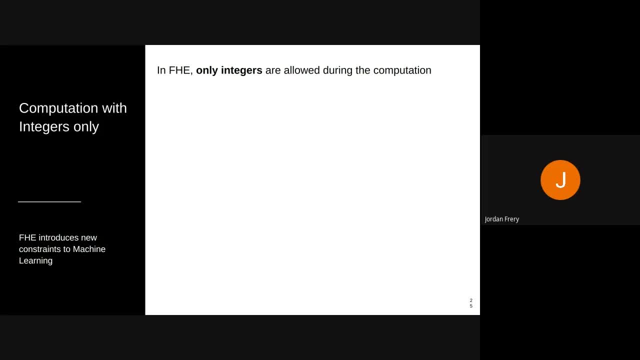 friendly. So in FHE At least- FHE At least currently- we can only work with integers. So computation have to be done with integers only, And to do this, quantization, we use quantization, which is an approach that allows transforming. 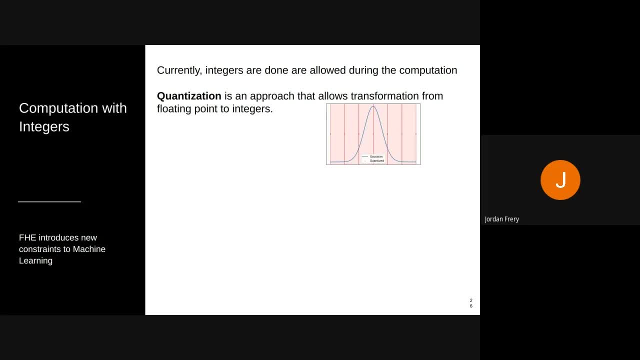 floating points to integers. So if you take a distribution like the equation distribution, you just cut the distribution with a full range. You can actually choose different Quantize if you want And you define a precision which would be like, for example, eight bits or four bits. 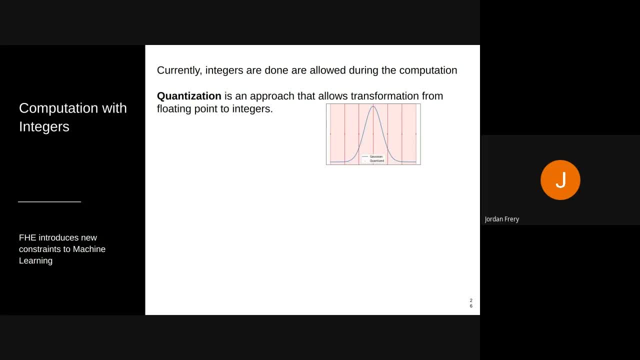 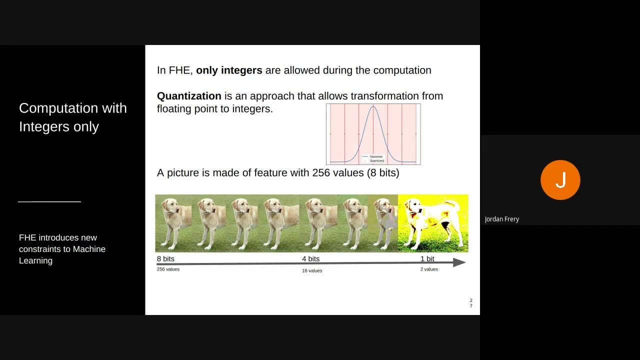 And you cut to your space into the number of available precision. A more visual example would be with pictures. Every pixel in a picture is represented with eight bits, So you can see that. So 256 values. If you would quantize the picture, you would see that you would lose some information along. 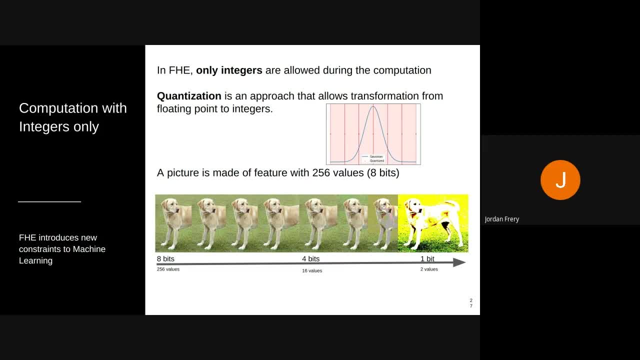 the way until you reach a single bits here which allows to have- Because there are RGB channels in picture, it allows to have some kind of a similarity. But if you would feed the right picture to a machine learning model, while it has learned over the first picture, 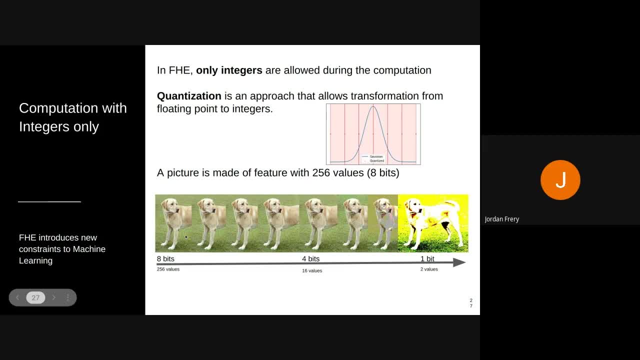 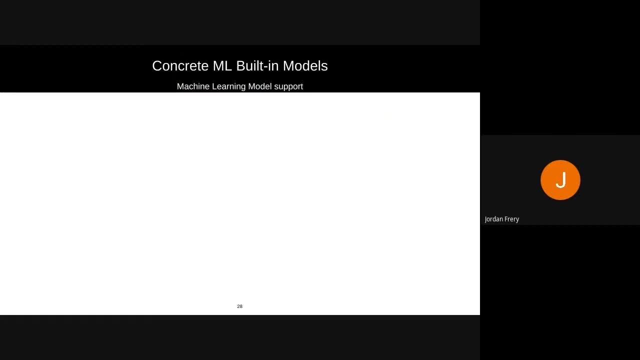 The eight bits one, then you would get some kind of loss in the accuracy. So let's look at what's available in concrete ML and what kind of machine learning model we support here. So the first kind of model: tree based model, So decision trees, random forest and attributes, which is a gradient boosting algorithm. 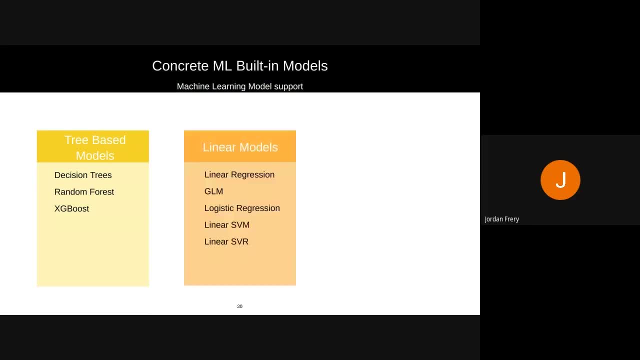 Pretty popular in machine learning. Then we have linear models. So basically linear regression, generalized linear models, logistic regression, SVMs and overs And finally overs that appear here, SVM, elastic net, lasso, reach, And then finally we enter the world of neural networks. 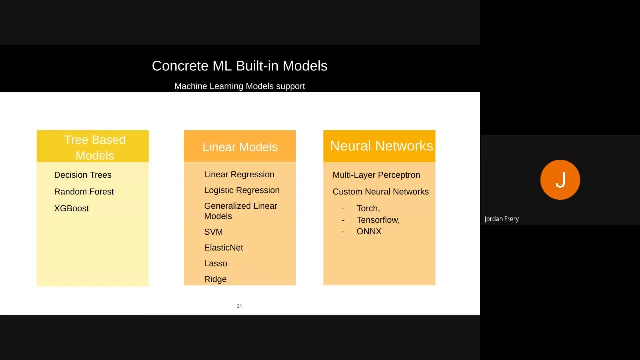 We have built in neural networks such that user can. And then, finally, we have built in neural networks such that user can- There's a lot of things. And then, finally, we have built in neural networks such that user can. And then, finally, we have built in neural networks such that user can. 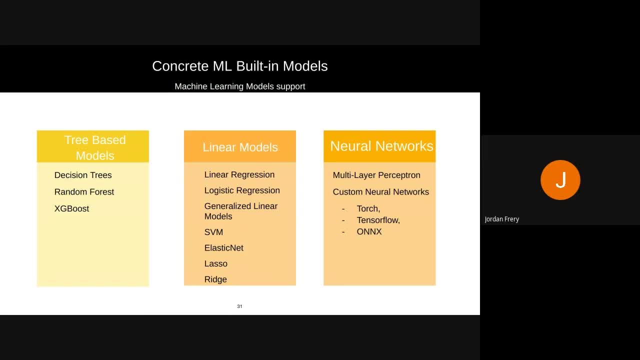 So we can actually train the neural nets, and the neural net is going to be converted to FHE instantly. Or we can also design the neural network using Torch TensorFlow, ONNX, if you will, And once the neural net is learned you can basically push that to concrete ML, which 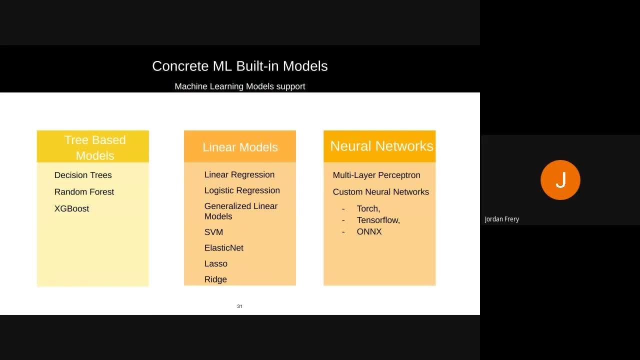 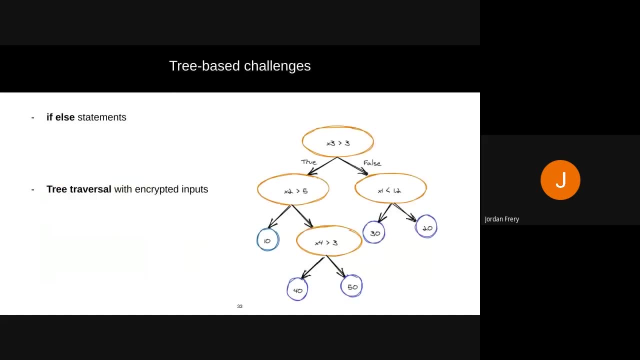 will do the conversion to the FHE equivalent. So let's take a look at tree based model here. So tree based model have a challenge which comes from the fact that they are built with if health statements. So in a tree traversal with encrypted input you would have to do comparison between the 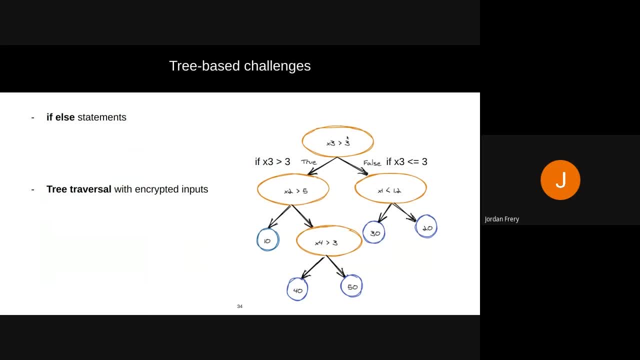 for example here the X3, which would be encrypted, and a clear value which would be in the clear with this kind of thing. But comparison Doing a greater than is not directly possible in FHE right. So what we do is representing this comparison with a table lookup. 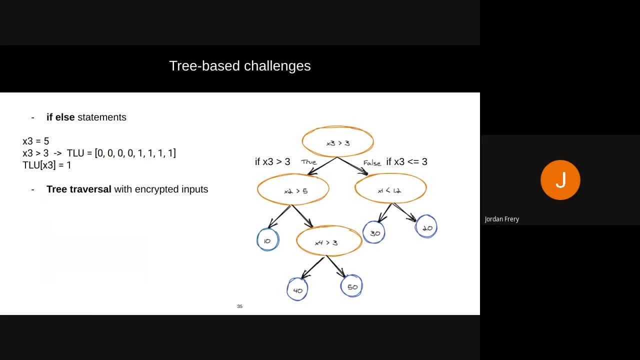 So imagine you have X3 here, which is equal to five. So the comparison X3 greater than three could be represented with a table lookup with only those zeros, four zeros and four ones. Okay, So what it means is that, like so here X3, you would just pass the X3 as the index and 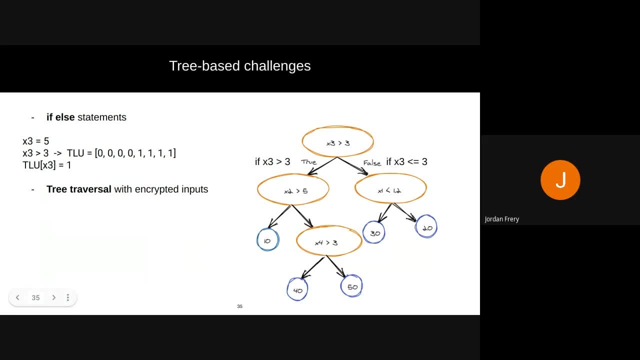 it will return whether it is actually greater than three or not. So this is essentially how we can do comparison in FHE now. So the second part is tree traversal. Okay, Tree traversal. assume that the example is only going to go through the nodes. that satisfy. 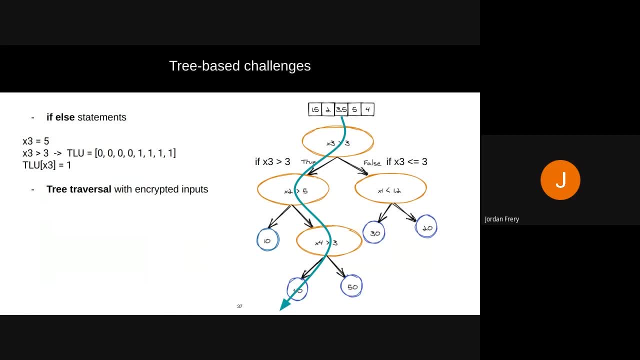 the condition. Well, this in FHE is not directly possible, because FHE, like in FHE, the input is encrypted. You can't really know, the server can't really know whether it has to execute the left node or the right node. 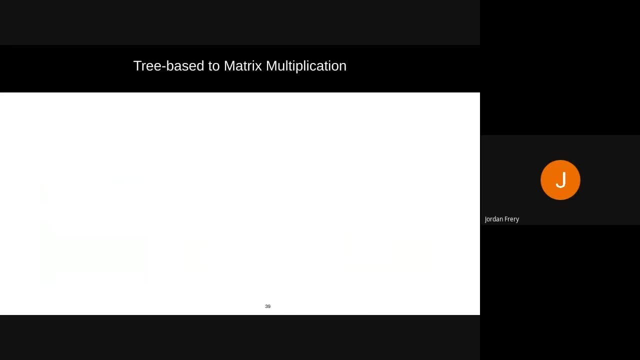 Okay, So. So we have to execute to process every single node in the decision tree, And we do this by basically converting the tree traversal model, like inference, to only matrix, multiplications and comparison, which we can do in FHE. So with an ONNX graph it would be represented like this: 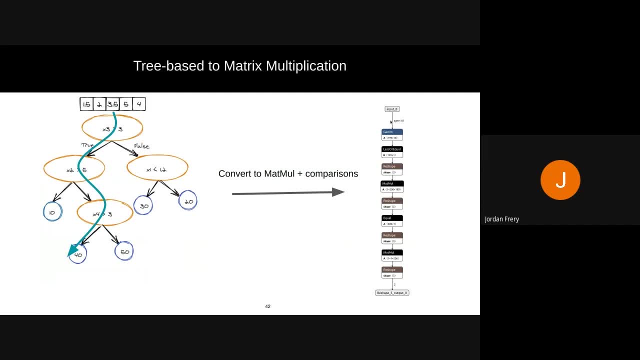 So we have a single straight graph of computations that computes every single comparison and every single condition in the tree. So this works fine for also a lot of different trees as they are in, like random forest, for example, or gradient boosting, as it basically just adds one dimension to the matrix multiplications. 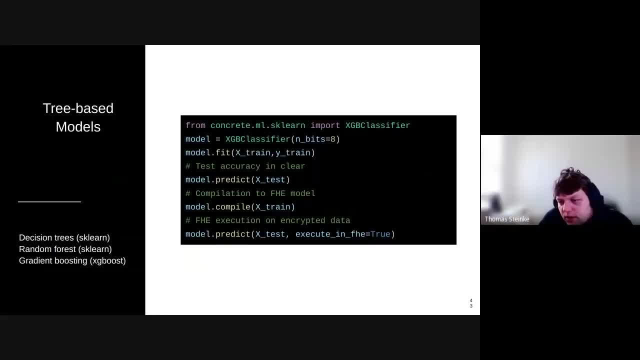 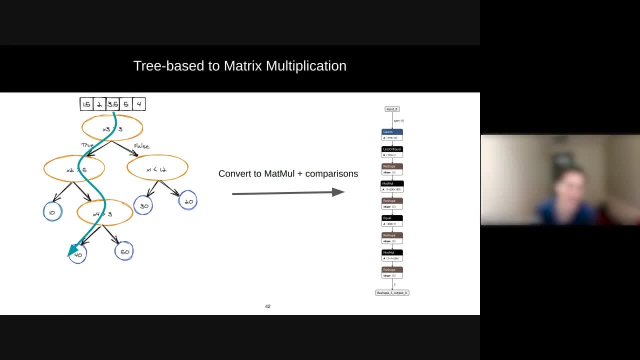 Great, Okay, Thank you. There's a question on the previous slide. Oh yeah, Sorry, Sorry, Yeah. For these tree-based models- and I think this question applies to a lot of other models- was there any alternative of like converting the? 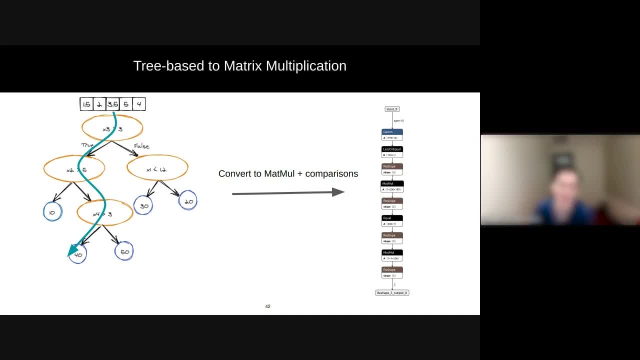 So, like the problem with these trees is if they're very deep, but if you're doing like random forest or something, you have shallow trees, you can sort of take advantage of parallelism. Was there an attempt to like rewrite these trees in a different form that makes them? 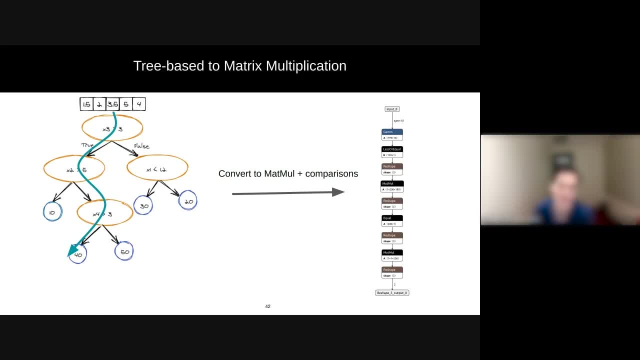 more suitable for the limitations of the tree? Yeah, that's a good question. Like random forest, for example, they're going to be so deep that if you don't constrain them to stop at a specific level, then they're going to explode in terms of matrix dimensions, 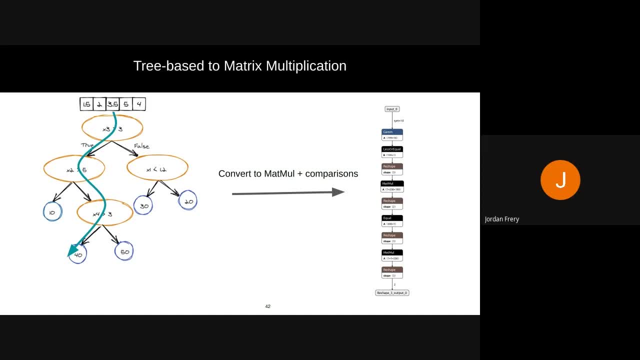 here. So we didn't really study ways to make the random forest the entire model with only small trees. But gradient boosting, for example, is basically the inverse. You've got some shallow trees and you basically combine a lot of them, but very, very like. 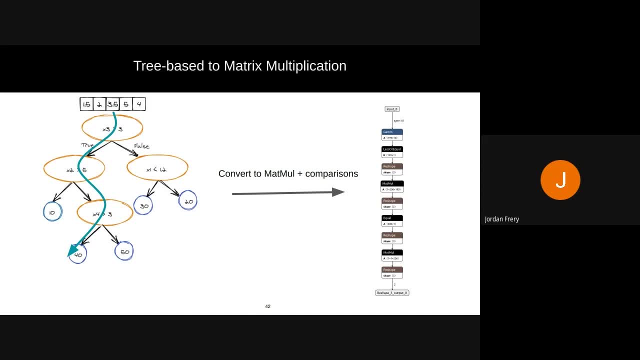 not deep at all. So here it's completely fine for FHE. but you're right, random forest in their default mode would be huge matrices here. Yeah, So I'm guessing this approach is probably taken to get all of the trees in the tree. 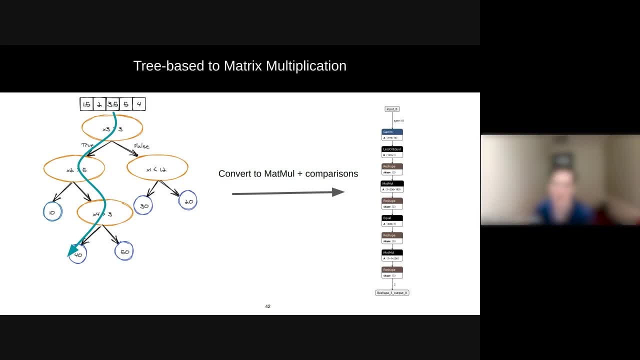 Yeah. So it's like: is it possible to get all of the models into sort of the same TensorFlow graph input type of format so that they could be sort of uniformly processed, Or is there like special handling for each of the different types of models? 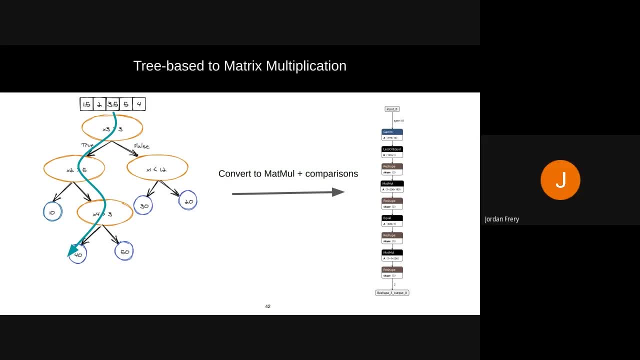 I don't know. So for tree based we actually use a library developed by Microsoft called Ehrmingbird which takes any kind of tree or ensemble of trees and transform these through the model And transform these to the matrix multiplication representation. So basically any kind of tree based algorithm in machine learning would be represented with 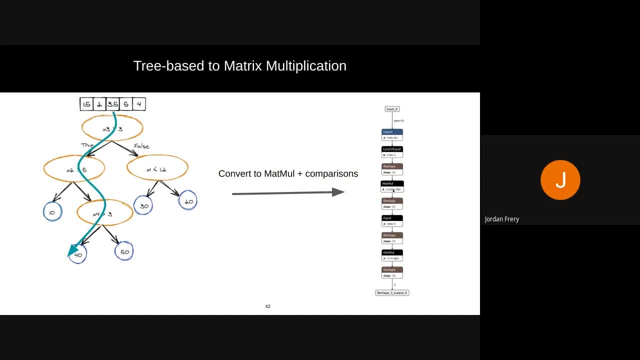 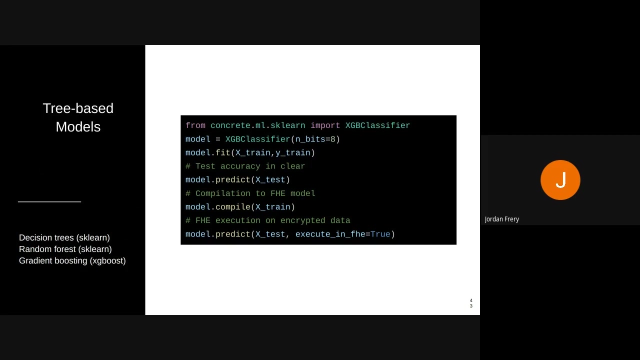 those nodes, Only the dimensions and the values to compare with would change. So yeah, Was that the question? Yeah, Thank you. Okay, Cool, Okay, great, Okay, Okay, Yeah, So Yeah. So the way we use concrete ML to develop a model, to train, model and predict and stuff. 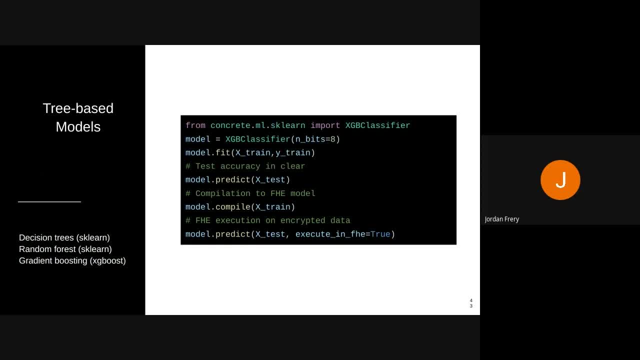 like. that is very similar to what we would have, for example, with CKIT Learn. So you just import a model which we chose to give the same name as they are presented in CKIT Learn or in their own library. So you just define the model. 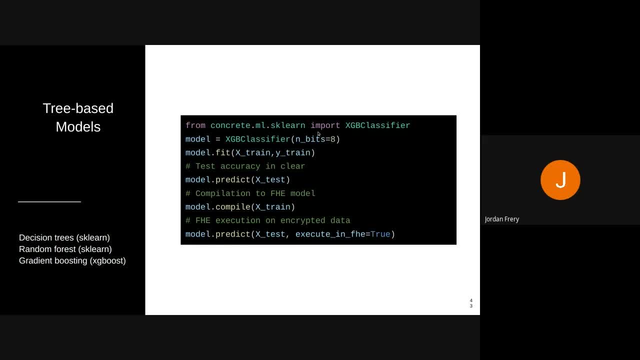 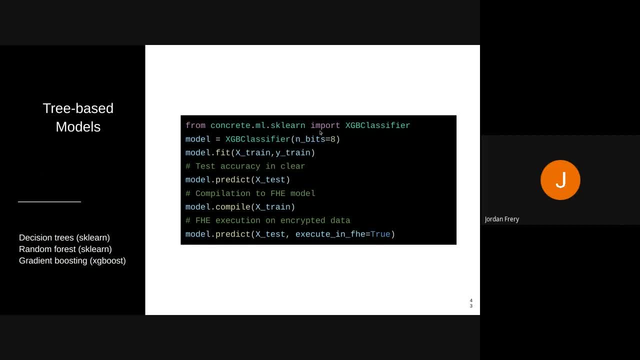 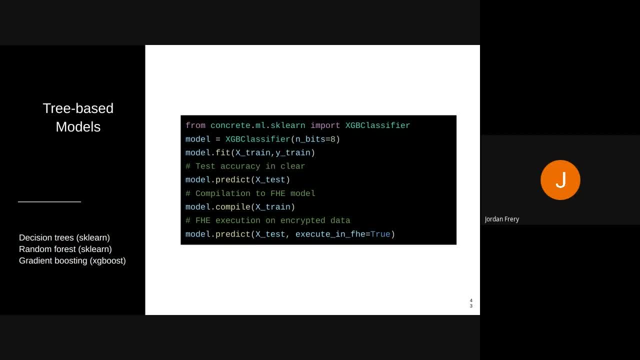 256.. While for neural nets you would have to quantize the whole input at once, because of course you send a lot of different inputs into neurons, and doing different quantization while then doing addition and multiplications on those differently quantized inputs would be very 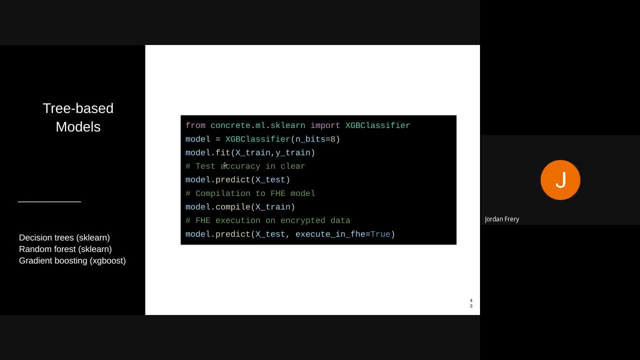 tricky to handle. But here, yeah, You can just train the model, So you define the NNBs. You can train the model with the fit function, then call predict, which would run basic, clear inference, So you can actually test, debug the model, compute some metrics which here would be. 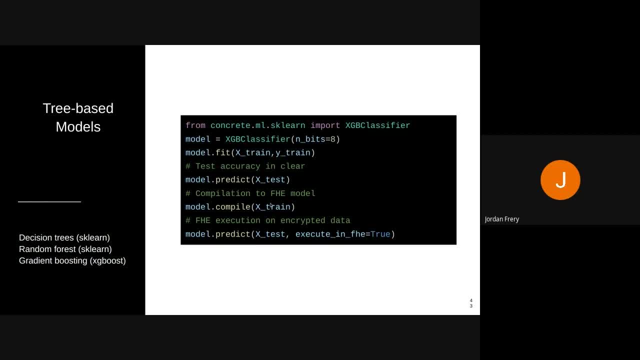 pretty fast because it's just everything clear. But it will give you the FHE accuracy because we run. we make sure that the cryptographic parameters allow you to Have something like one over 100,000 chance to give the wrong output. So then you can just compile the model. 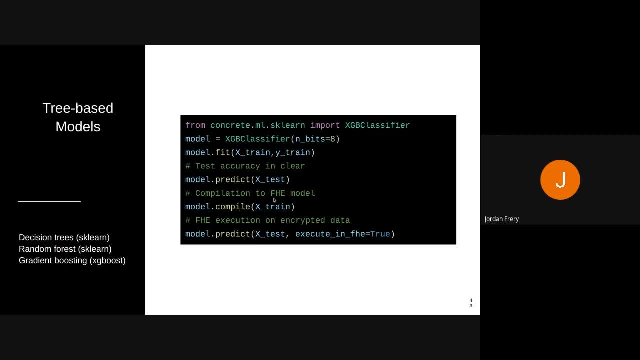 This compile function is going to take some representative data set and transform the model into different steps until it reaches the compiled. So we have a MLIR representation of the model And then, And then, And then we can basically execute FHE operation, pure operations- following this MLIR. 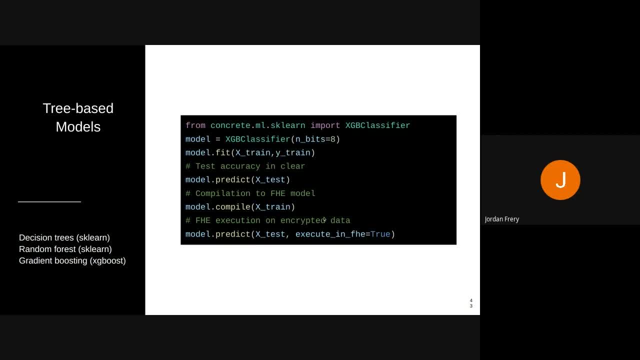 And yeah, of course you can check the execution time by just simply setting the executing FHE here. Of course, XTest here is not encrypted, It's just for debugging purposes for data scientists, But then you can. once you are ready, you can just split the client and the server. 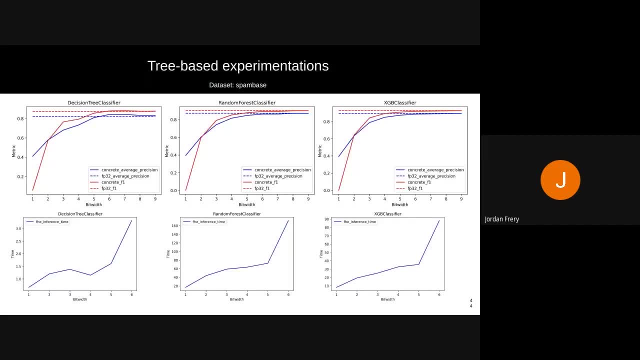 And then deploy basically. So those are a few experiments of a spam based data set where we take the floating point for two metrics, So we have the F1 metric and the average precision metric- and we compute the metrics for different. So between it would be the end bits parameter that you just saw before. 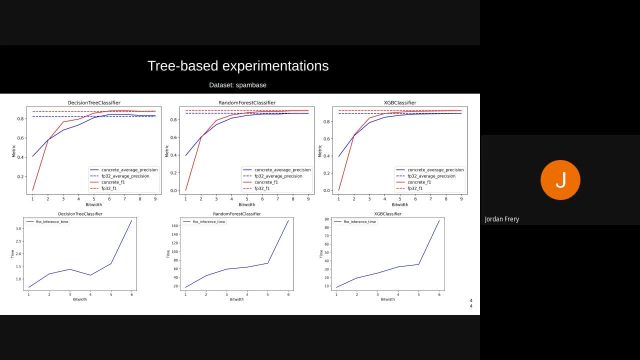 And of course we've one and two here, Yeah, And then you can see the damage done to the accuracy of the F1 and the average precision is pretty, pretty huge. But you convert very quickly to the floating points: 32 metrics, which is, which is great. 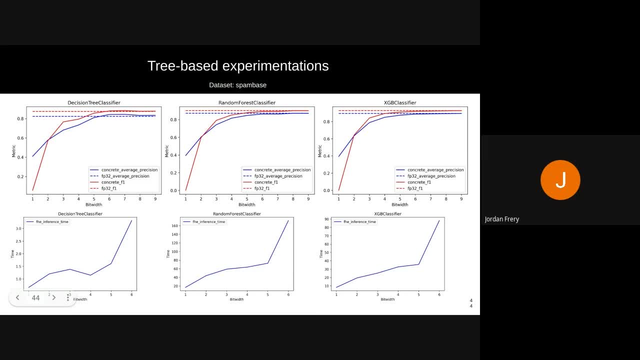 And on the bottom you can see the inference time for a single example. So of course, here I probably would need to give you more information about what's the size of the random phrase. It was in this interest, But yeah. 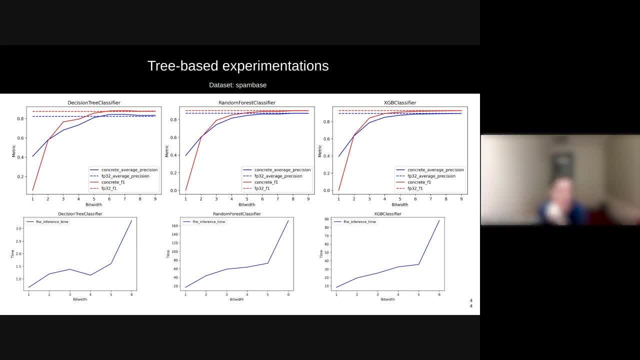 On time here. knowing FHG, that could be minutes or seconds or Yeah. yeah, very good point. So those are seconds, Those are seconds. We. we basically here use the default parameter we have in concrete ML. I think there is no depth limit for decision trees. 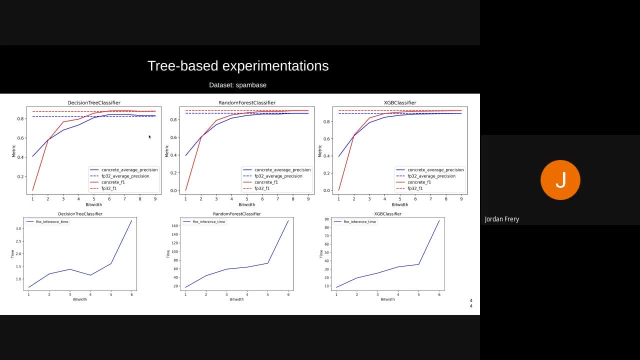 There is a depth for XGBoost and I think we set six of depth running for us. So decision tree, of course it's a single tree, So it's pretty fast, But you can see that from one to six it will triple in terms of execution time. 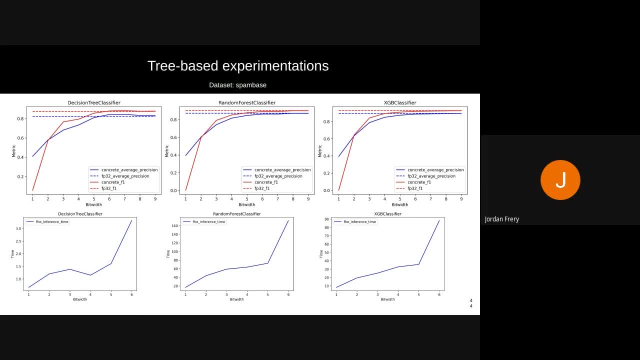 Random forest, as you guessed, is the most costly of the tree based model because it just builds very deep trees And XGBoost has a. I guess it's more friendly to FHG because it builds very shallow trees while having good accuracy. Did you say how big the decision tree classifier example was? for like three seconds. 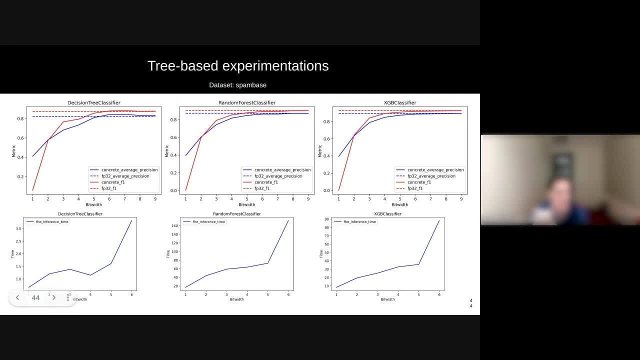 Like roughly, how big was the resulting network or the tree that started? Well, yeah, So we don't set a limit on the depth, so it will very much depend on the data set. I can't really tell you. It's a very good point. 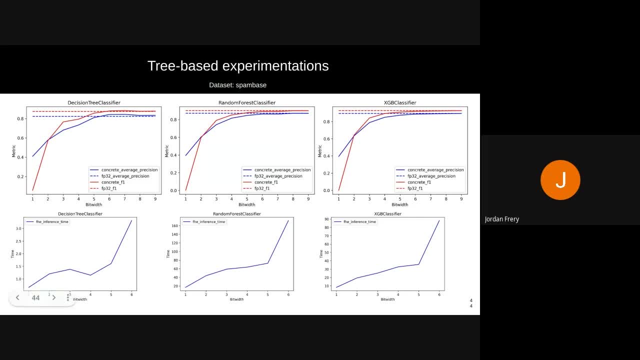 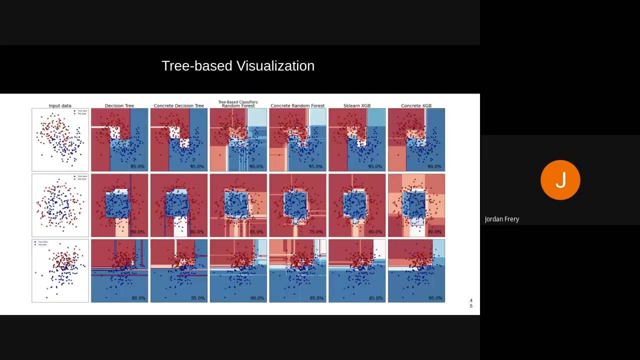 I should actually write the complexity of the models here, But yeah So, it's basically trying to classify The span base training sets properly, but it's a single tree, while we have 100 here and 100 here. So, yeah So, and there are a few visualization graph. 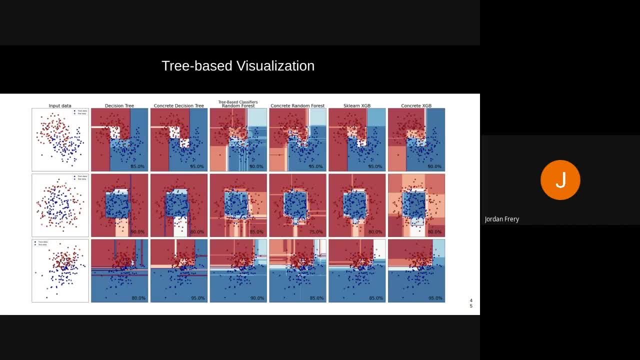 Just to show that, even though the decision boundaries are not set at the same place, because of course we can't size them- But that's what people were saying about the output space- I will So basically quantize the output space entries. 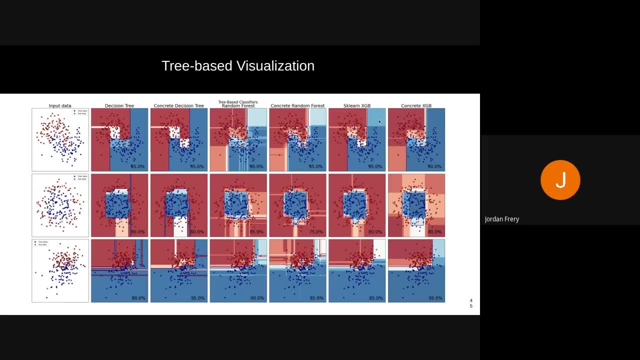 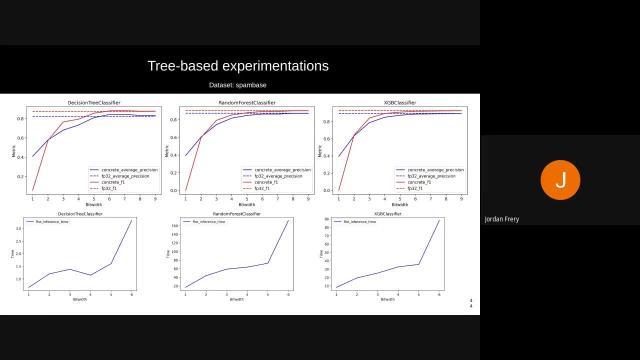 Well, they also in your nets, So. so you have got some different kind of decision boundaries, but the results are very, very similar in the end. Oh, and something I didn't mention before, but we see some kind of an effect that we didn't really expect before. 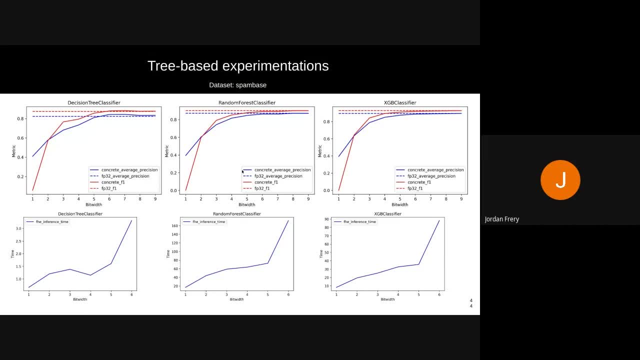 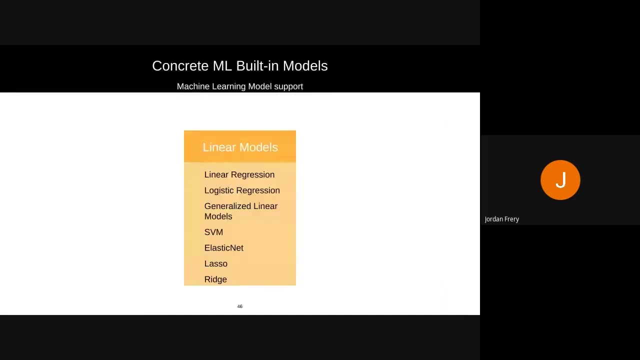 Like when running. that is, that quantization has some kind of regularization, Yeah Yeah effects here, where, like, the concrete has some kind of better accuracy for a moment, just because quantization makes data less precise. so, yeah, great. so now linear models. so we have a few of them. 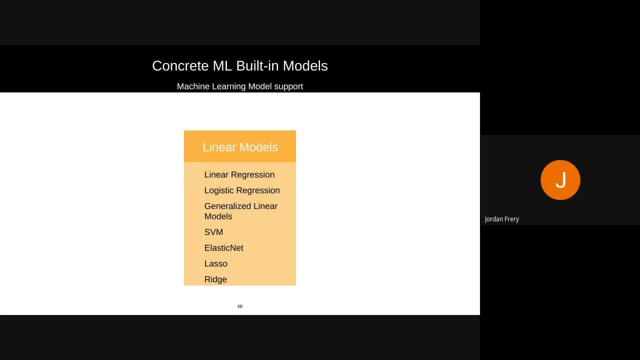 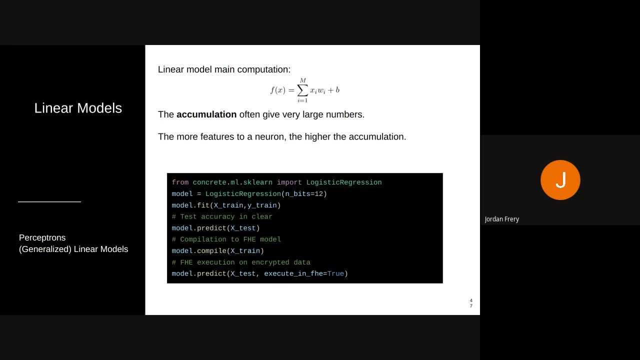 we basically tried to cover all the linear models that were implemented in secret: learn um. the good part here is that it is what it is what we call leveled fhe. it's a circuit in fhe circuit which does not contain programmable bootstrapping. what this allows us is that 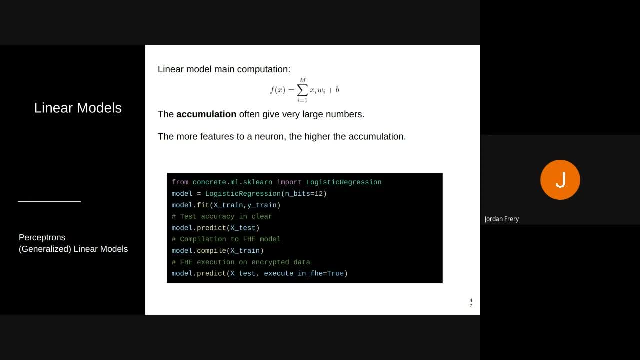 we have a, we have a condition on programmable bootstrapping. that i didn't say before is that we cannot go over a certain number of bits of precision. uh, so i can give you an example: like a year ago we were at around six bits for um. 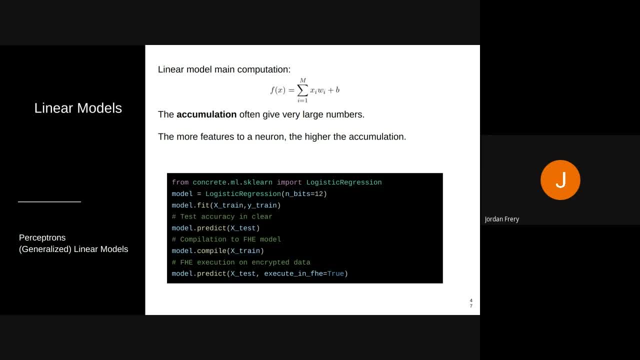 the input of a pbs. it couldn't go over that. i went to seven, uh, eight very quickly, and now we are at 16.. so the accumulator cannot go to 32 bits, but we we've got like 16 bits, which is um, quite, quite. 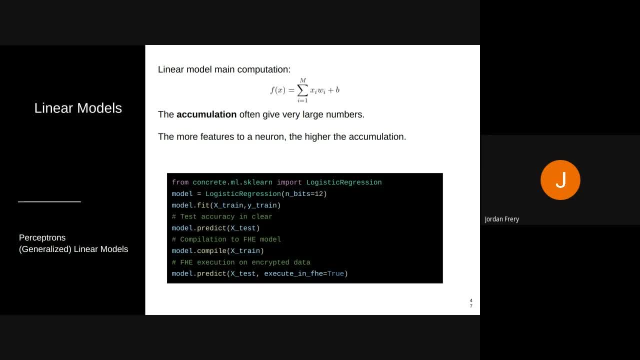 good. but this does not apply to linear models because there is no pbs. so here you can do very large some uh. we can go up to 30 bits. so for example, here the number of bits we have is a quantization on the input but also on the weights. so you're gonna do like uh, 12 bits, um 12 bits, uh times, uh, 12 of the bits. 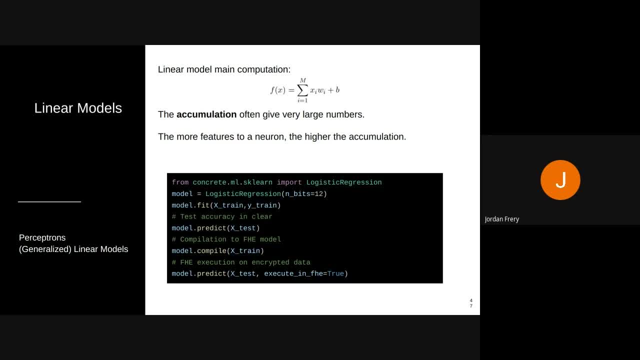 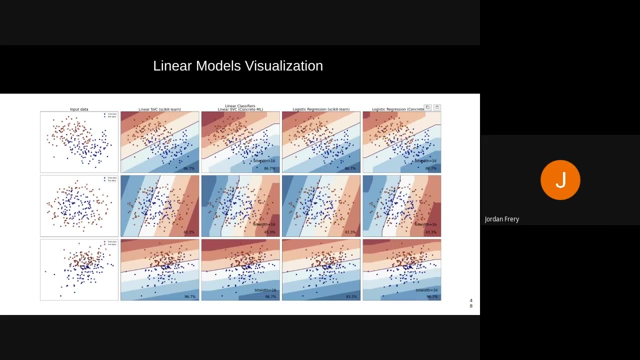 and then adding a bit bias, so you're gonna have some really large precision, uh, really large, relatively really large precision in the accumulator here. so essentially this allows us to match um the floating point 32, um accuracy, but also the run time. is is just uh, super fast. we just match uh. 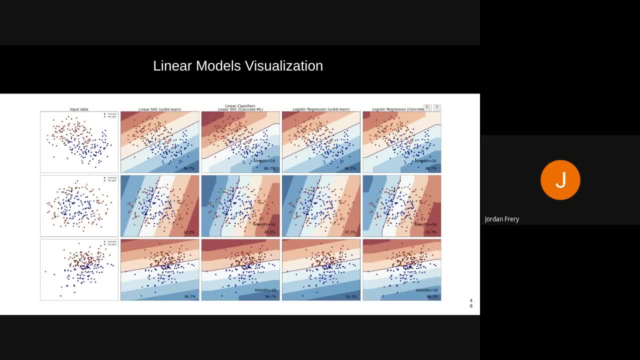 um by it, by another of my radio, of course, uh, the floating point 32, um execution time. uh, in this visualization you can see that, uh, while we are in the input range, the model behave quite similarly as the one on floating point 32.. you can maybe see, like the artifact, like the, the fact that basically, the 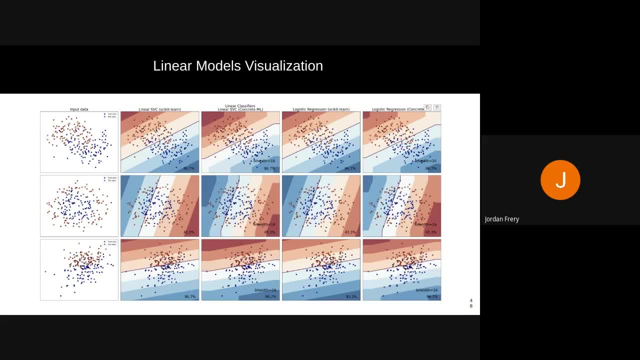 quantization makes the out of bound like out of range input. that is, just without any value. so in this case, you can see that it's uh, it's basically uh going to overflow, and this is not something we want. that's why, when you compile a model, you would want to give an as a representative input. 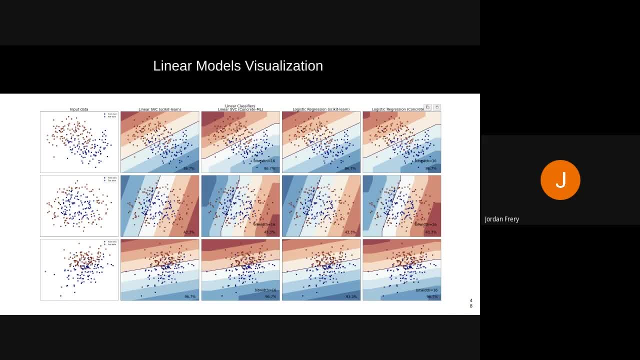 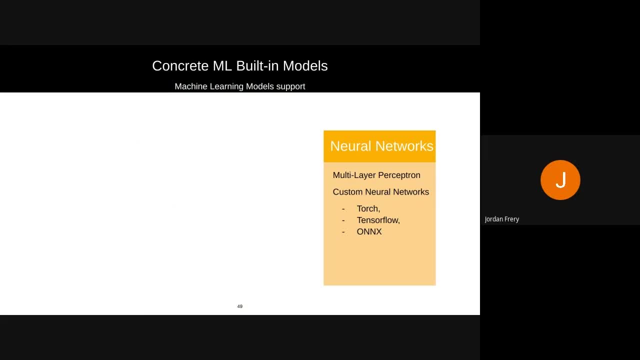 data point, like as possible. and now comes the last part. so neural networks, uh, the first thing is that we have built-in neural networks, so essentially, just a neural net classifier, neural net regressor, right, um, you can see, it gives things like that. so, as i said, 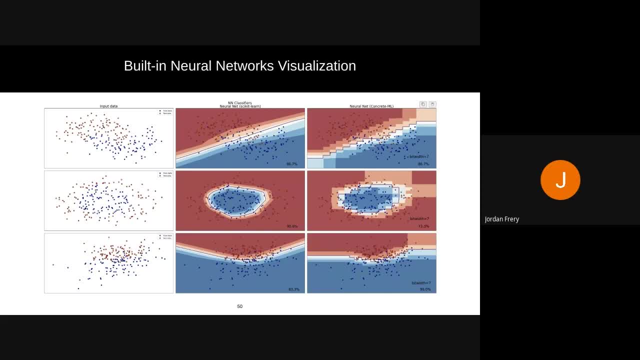 one complexity with neural nets is that they do very large multi-sum and then there is a pbs. so it's not like linear models. we can just have very large uh precision. we have to make this the accumulator. so for every single neuron you are in the neural net, you have to make the accumulator. 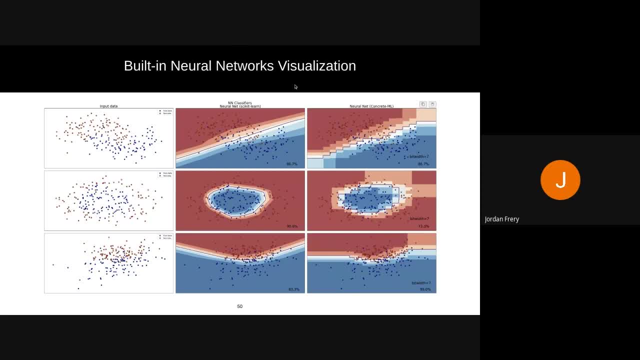 less than 16 bits. so you can do this by either quantizing the inputs over lower bits, or you can apply different kind of regularization to make the accumulator remain around zero. there are a lot of different ways where you can also basically just break the, the matrix multiplication into several. 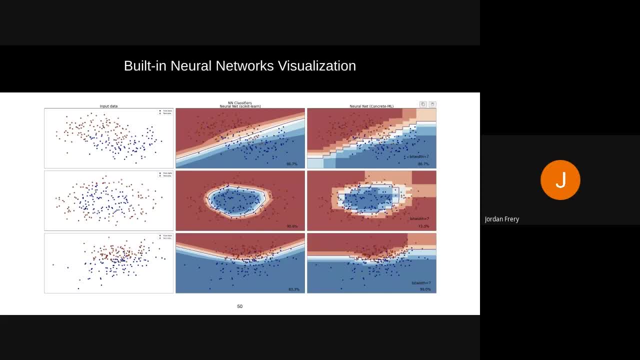 different matrix multiplications. but yeah, the main point is that the accumulator must not go over 16 bits to be able to use it in a pbs. so here you can see the quantization boundaries, which are much less smoother. smooth, uh, smooth that. and then the floating point, of course. 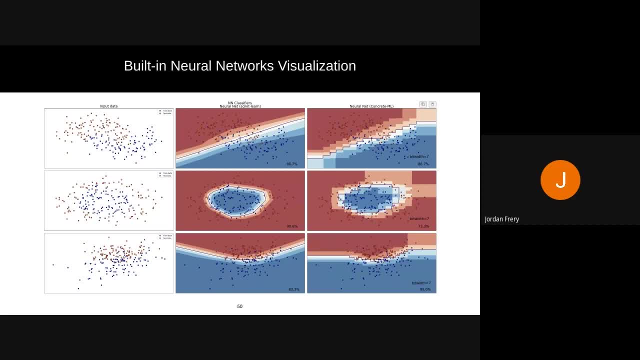 but the, the, the, the accuracy remains, remains, uh, stable, um, here to train the neural nets and make it like quantizes it we are. we have kind of two different ways to do this. one is that we can use different ways. the first way is training on your net network and just applying what we call. 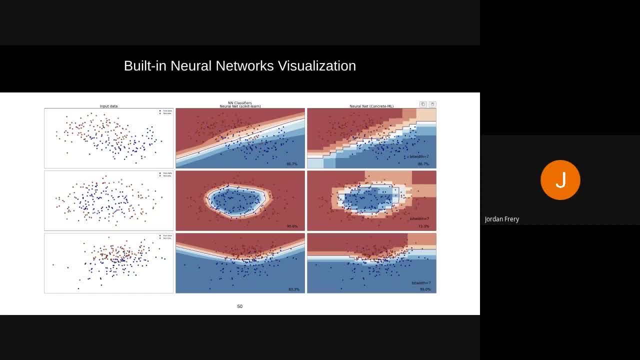 post-training quantization. in this kind of quantization you just naively: take the input, quantize it, take the weights, quantize it and that's it. you don't do anything else to your neural net. of course you would calibrate the activations, but once it's done, it's done so. 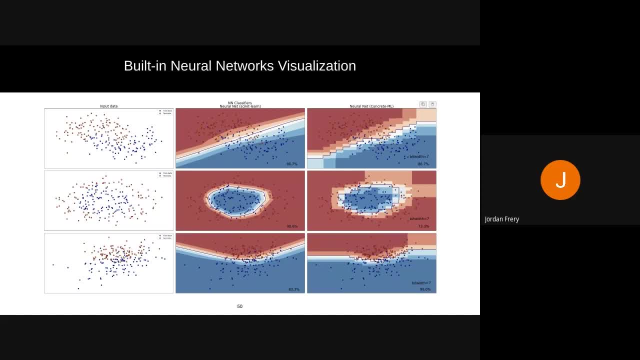 here to have a bit more accuracy. we use quantization aware training, where during the training of the neural net you fake quantization. so in the inference part you apply quantization to the weights and to the activations, also the inputs, and so the neural net sees only. 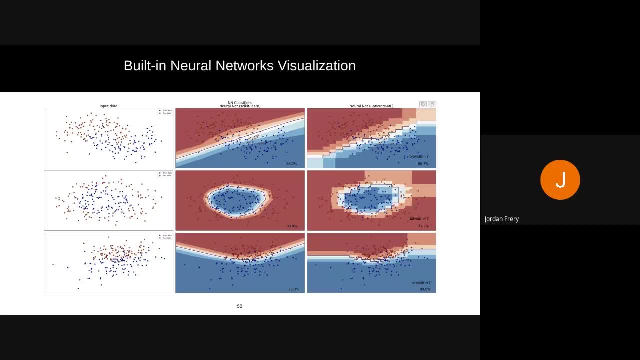 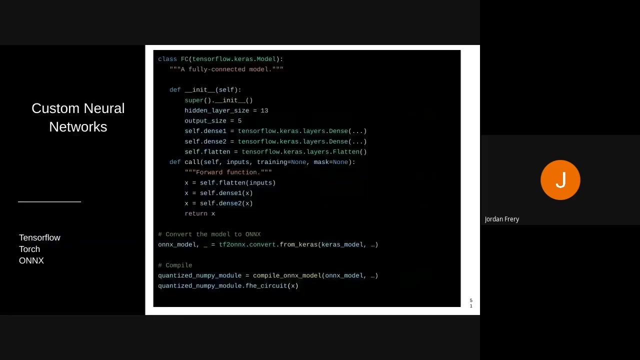 n bits of precision, and then you apply the gradients over the 14.32 weights of course, and that way you can converge to a much better solution, which make the final neural net great. with great accuracy we found the integers. the second part is one that we are actively developing. this one is: 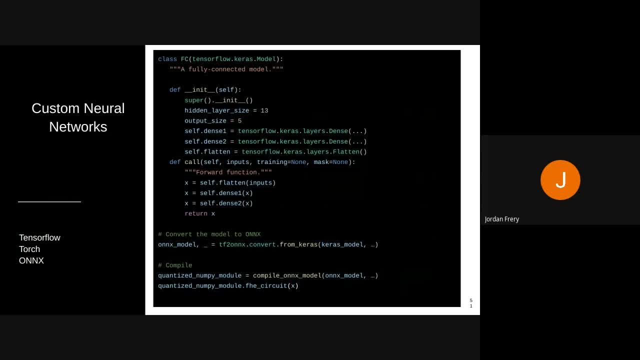 developing a custom neural network so you could take uh, for example tensorflow, and create a like for example here, a fully connected model. so you can do whatever you want in the, in the, in the model uh, with the exception of a few operations that are um, that will be available soon but very costly in fhe uh. those are, for example: 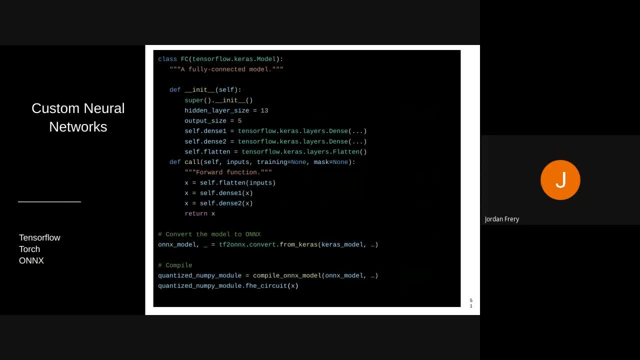 for example, ranking or doing something like max pooling, which are costly operation could be done, but a bit more costly, and so the first step is so you basically create your keras model- let's say it's fully connected here. you transform it to onnx, so there are different libraries that actually do this. 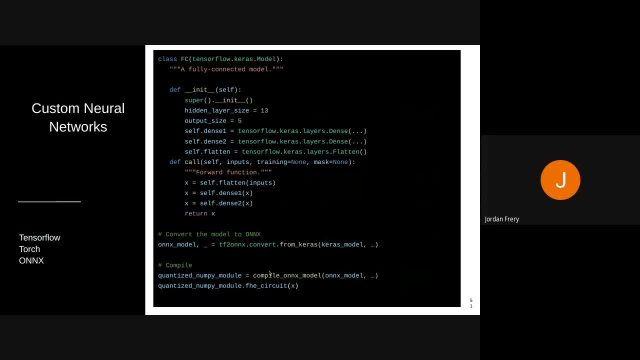 very easily, and then you can just send this into a concrete ml function, which is called compiler and next model. so here we take the graph, we transform it to um, to numpy functions, and then we use uh, another open source library developed by zama, which is called concrete numpy, which essentially um convert any numpy. 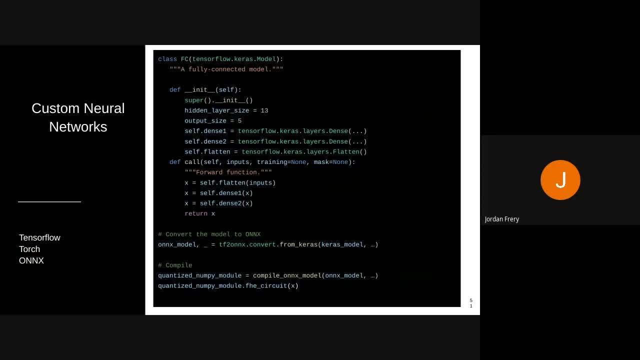 functions to their morphic equivalent, and then you can simply, so you have a quantized module here returned by concrete ml, and then you can call this fhe circuit that can run over encrypted data and of course here from from there you can also split server client and deploy easily. 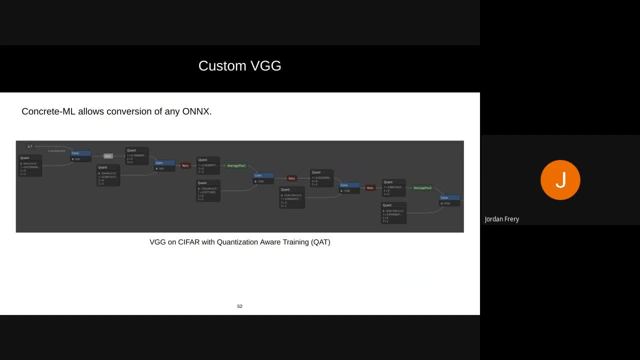 so, um, we recently developed this for a vgg-like network using quantization aware training. so if i plot this into a graph representation using the onnx format, you'd see that in the graph you have some quantization node appearing. that will be very useful for us because we're gonna take the, the parameters of this quantization. 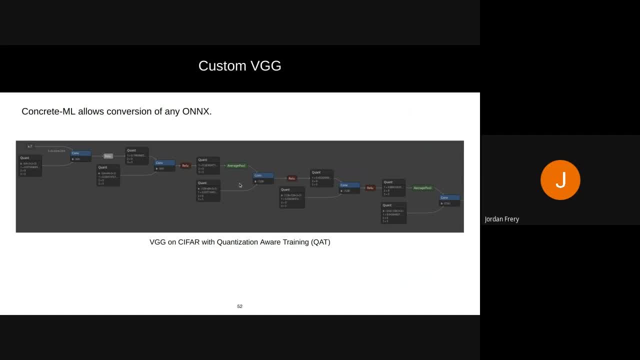 and and simply apply them such that now the weights and the results uh, at every output of quant nodes uh will be integers. so in the end, what happens is that the output of the convolution can be, so must be, remain, less than 16 bits. and then we make the relu, the quant node and the 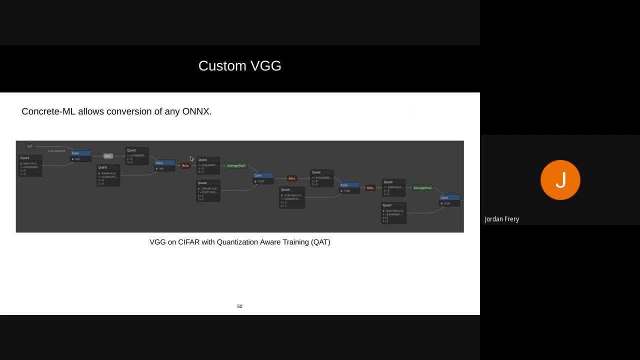 average, pooling a single pbs, a single pbs for every output of the convolution, of course, but we, we fuse them together, uh, and so, basically, pbs takes the output of the call and then the output of the of the pbs is uh going into the another coalition, and so on until the end of the network, um, where the output can be um. 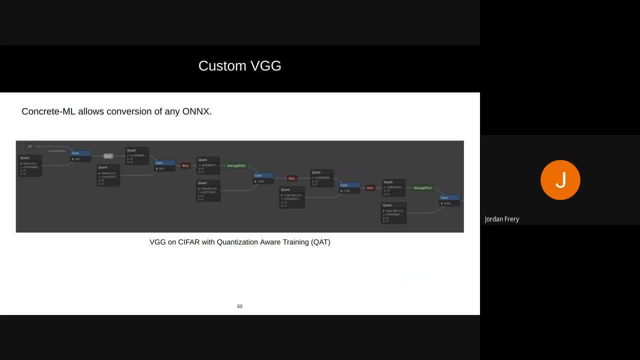 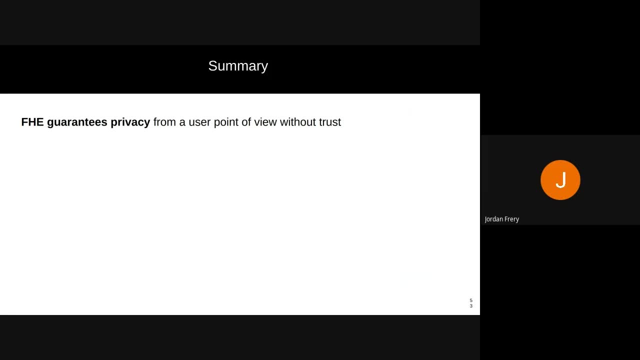 decrypted by the user. um great, thank you. so fhe guarantees privacy from a user point of view. uh, the main, the main thing here, i think, is to remove trust from the process of the user asking a service to a third party, because trust is not needed. the server is actually just selling a service and the user wants the service. 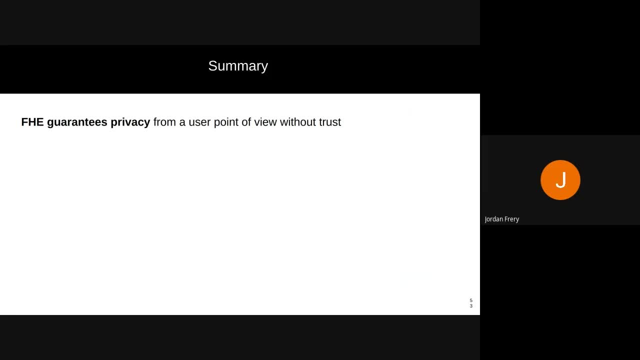 the user just shouldn't have to trust the server that it's not gonna leak the data or whatever. actually, even for the server it has an advantage because data leaks are very happening, very often even though it's not actually the real of the company. quantization is an heavy part of our open source library, which is a necessary step. 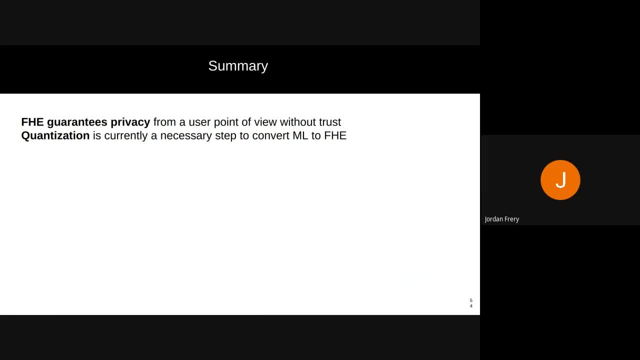 to convert machine learning model to the fhe equivalent. we have three base model and three linear models which are very accurate in FHE. So of course, if you take a random forest and try to have the largest random forest, you're gonna have some trouble. but for example, XGBoost models, they 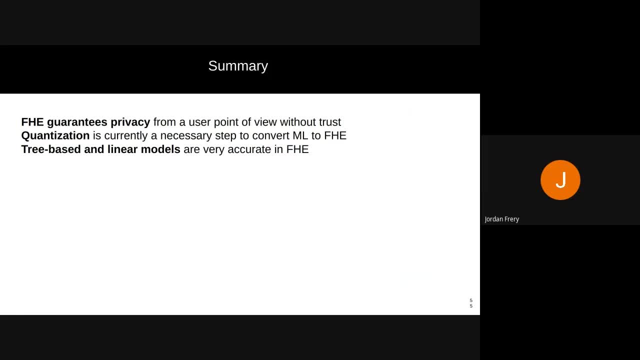 perform really well with shallow trees and give some very accurate results. so and linear models are just very, very close to their F floating point. 32 equivalent Neural network can be more constrained. these all come from the fact that the accumulator even in quantization real. in the research it's very often assumed that accumulator are not quantized, so even 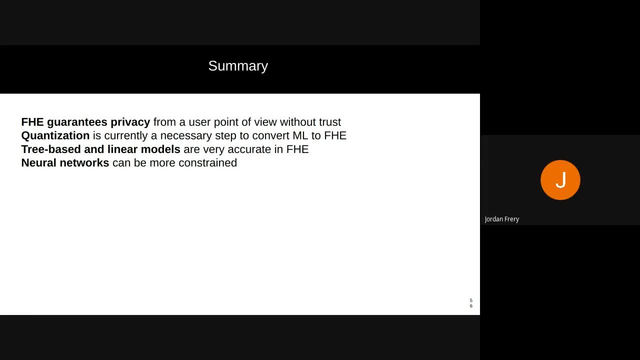 though they quantize, even with low bits, inputs and weights, they just don't quantize the accumulator. so they have a 30, 32 floating point accumulator that is freely available. Other parts also mentioned that the input, for example the first layer of a neural net, 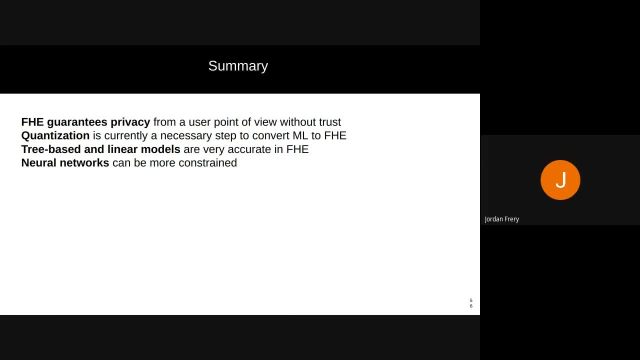 shouldn't be quantized, so they don't quantize it, while in FHE, we would like to have the whole model executed in the cloud rather than asking the user to do this. So no worry, ConcreteML is built for data scientists. we are trying to make everything. 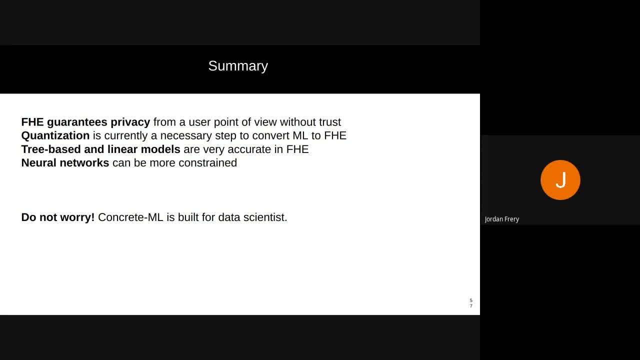 simple and smooth so that user can do the data. scientists can do a walk, their daily walk, and not care about cryptographic aspect of it. So there is a, of course, all the secret learn pipeline, like the grid search to optimize the model, all available. they are supported in ConcreteML. 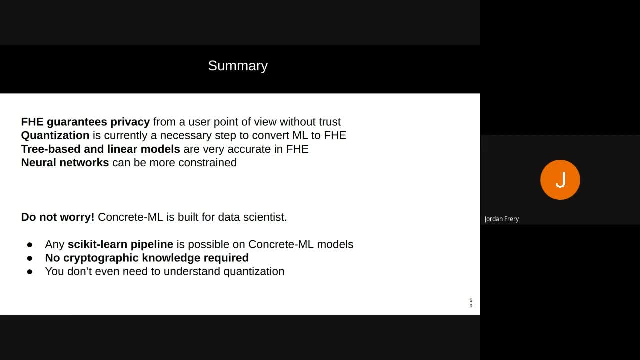 so of course no cryptographic knowledge required here unless you want to check how FHE is working behind the scene. you don't need to even understand quantization, at least for built-in models. if you want to do a custom neural network model, then you'll have to.